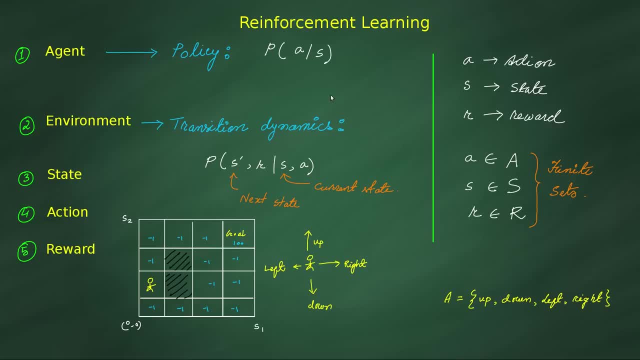 mathematical terms, because we will be using these terms to understand Bellman equation and policy iteration algorithm and value iteration algorithm. in our previous video about Markov decision process, we talked about the five components of Markov decision process, that is, agent, environment, state, action and reward. let's see what it exactly, what these terms exactly mean in terms. 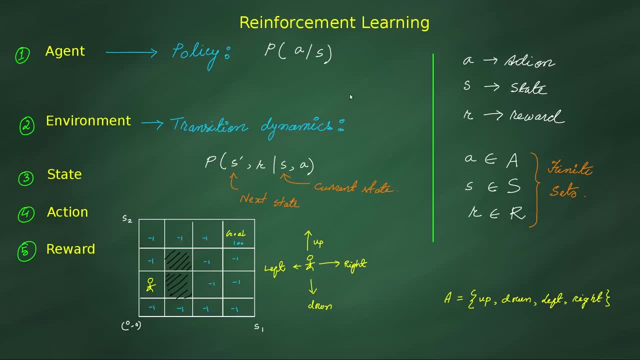 of mathematics. here the agent is a main decision maker. it has something called policy. policy is a function that map states to action. so you can say it's a probability distribution. it's a probability distribution of action, given a probability distribution of action, given a particular state. it can be deterministic also. it can directly map. 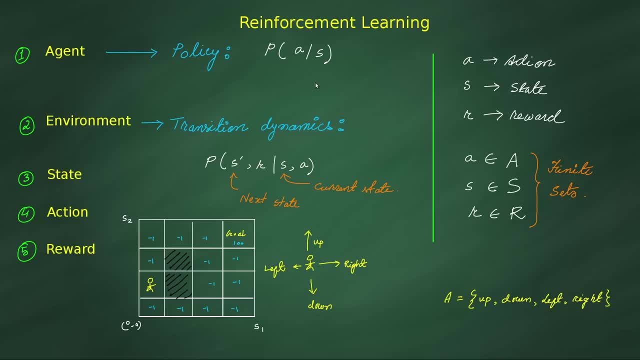 state to an action, then in that case it's, it, can, it will be a deterministic policy for the purpose of making it generic, so we took probabilistic policy, or you can say it is stochastic policy. and then the environment. so environment is basically the transition dynamics, how the state in the environment changes and how the agent. 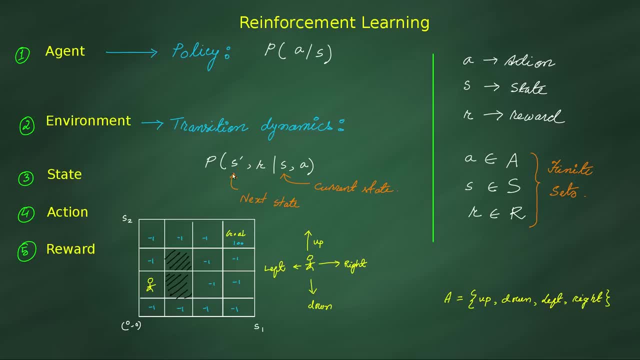 gets rewards, so it's a joint distribution of next state and the reward based on the current state and action applied by the agent. so it gives the probability distribution of next state and the reward. it's like a joint distribution. let's see this example. I have shown this example to make things. 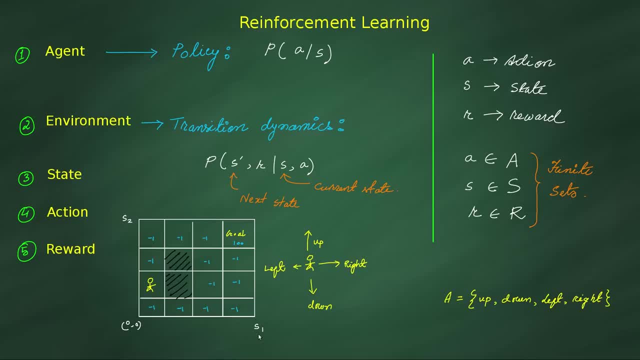 more clear. so here you can see these are the states. so it has two dimensional states. so state s1 and s2 and you can see the agent can have these four different type of actions up down, right and left. so what the policy will do, policy will tell the agent at a particular state like this. it is in this: 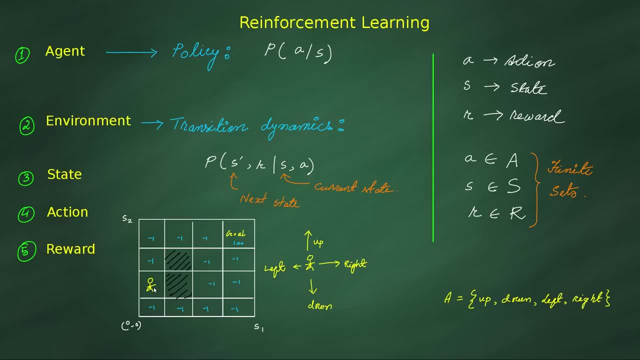 state what action to take to get the maximum reward possible in its episode, or finite number of steps in every state it gets a reward of negative one and when it reaches the goal it gets a reward of hundred. so you can see, if the agent takes this route then it will get more negative points than taking this. 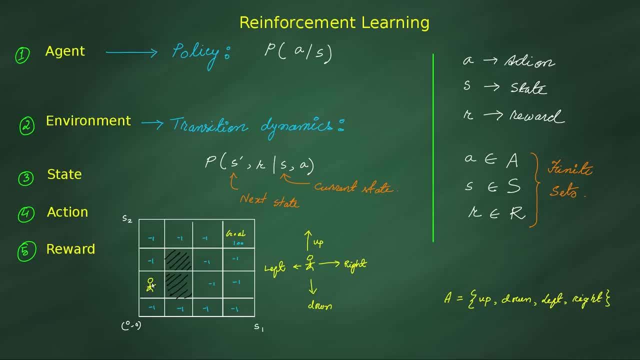 so what the policy will do. policy will tell the agent at a particular state- like this it is in this state- what action to take to get the maximum reward possible. uh, in its um episode, or finite number of steps. in every state it gets a reward of negative one, and when it reaches the goal, it 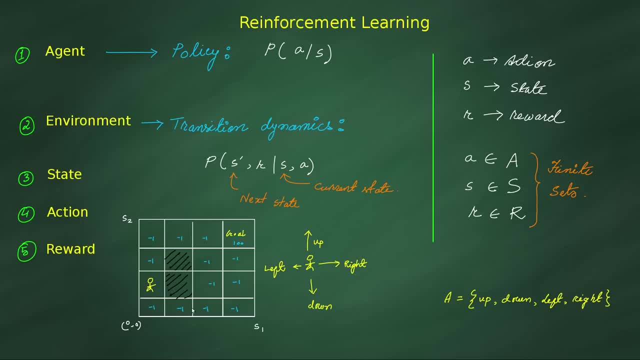 gets a reward of 100. so you can see, if the agent takes this route, then it will get more negative points than taking this route. so this is the optimal path. you can say this is the optimal policy. maybe, like in this state, the policy should say that it should go up up then, right, right, right. 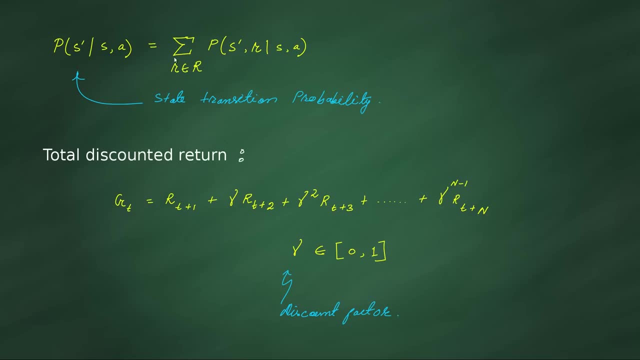 um, so let's go to the next slide. here we can also get the state transition probability from the uh, this joint distribution of state transition and reward. so how we can do that, we can simply add this: this probabilities for all the reward values. so just kind of marginalization. let's define a term called. 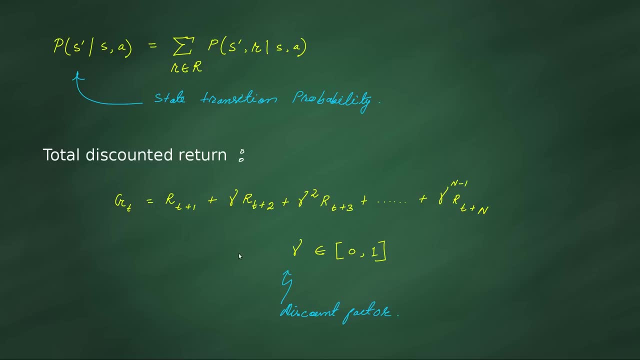 discounted reward. so it is the sum of the reward, but it's a weighted sum, weighted by a term called discount factor. so this discount factor is between zero and one. it is this decided by the programmer or the designer, and this term is used to give more importance to the 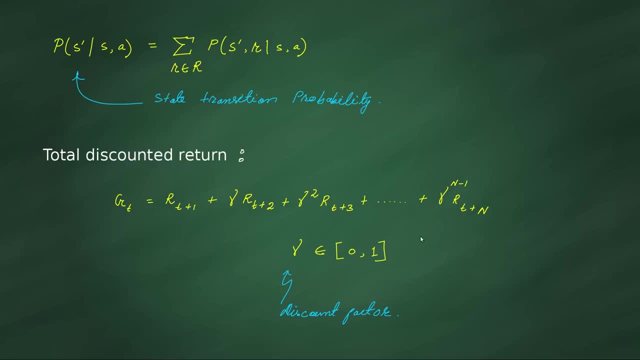 initial rewards than the very distant reward. so, like you can see, this term will get decreased when it is like multiplied with itself. so its power is increasing. so first it is power one to the power two, then to the part three. here it is, at the end it's to the power n minus one. 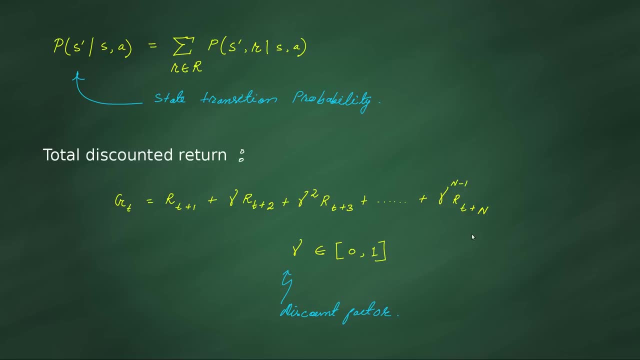 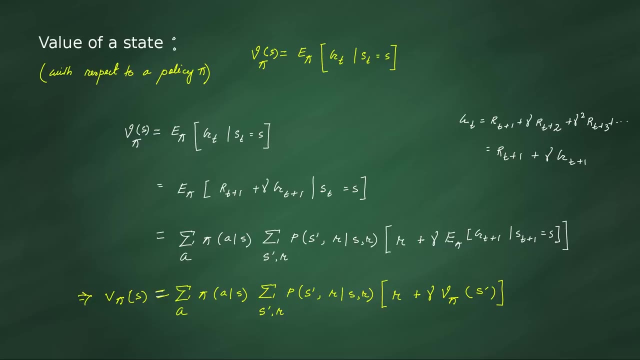 so it is giving less and less importance to the more distant reward than the initial rewards. so now let's define what is value of a state. it's the total expected discounted reward with respect to a policy. suppose you are in a state and you apply policy on the robot. 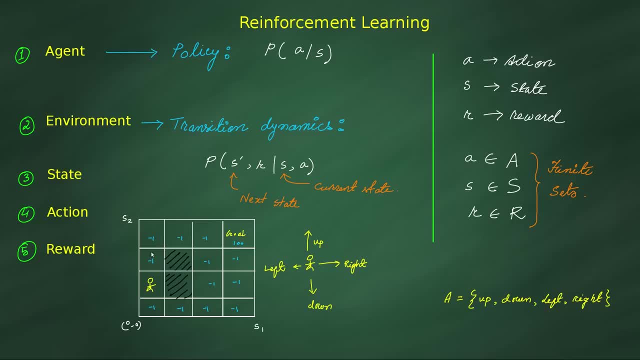 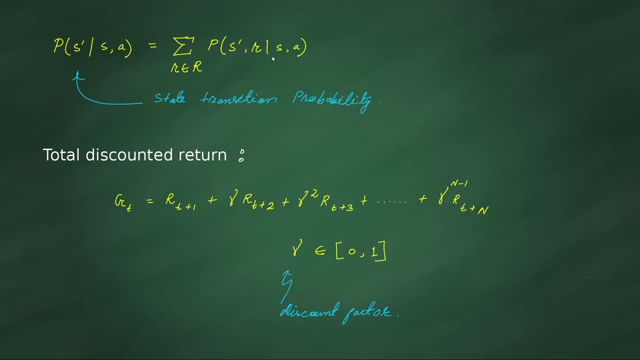 route. so this is the optimal path. you can say this is the optimal policy. maybe, like in this state, the policy should say that it should go up up, then right, right, right. so let's go to the next slide. here we can also get the state transition probability from the, this joint distribution of state transition and 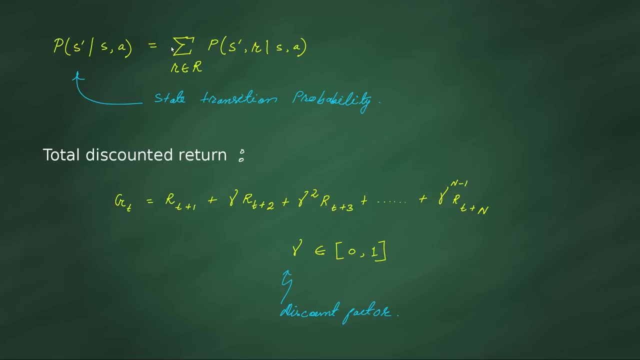 reward. so how we can do that? we can simply add this, these probabilities, for all the reward values. so just kind of marginalization. let's define a term called discounted reward. so it is the sum of the reward, but it's a weighted sum, weighted by a term and, as I mentioned in the last video, we that one is a. 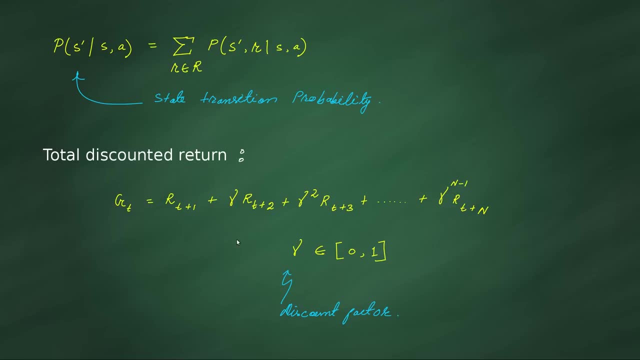 called um discount factor. so this discount factor is, uh, between zero and one. it is this decided by the programmer or the designer, and this term is used to give more importance to the initial rewards than the very distant reward. so, like you can see, this term will get decreased when it is. 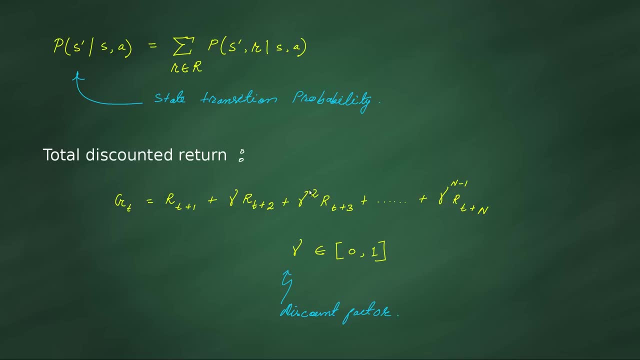 like multiplied with itself. so its power is increasing. so first it is uh to the power one, to the power two, then to the power three. here it is, at the end it's to the power n minus one. so it is giving less and less importance to the more distant reward uh than the initial rewards. so now 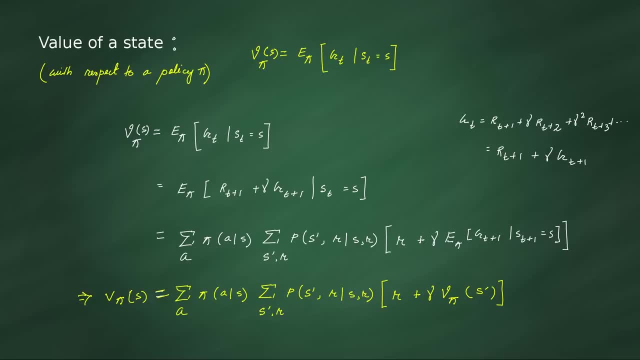 let's define what is value of a state. it's the total expected discounted reward with respect to a policy. suppose you are in a state and you apply a policy on the robot and you see what is the expected discounted reward and this is the value of the of a particular. 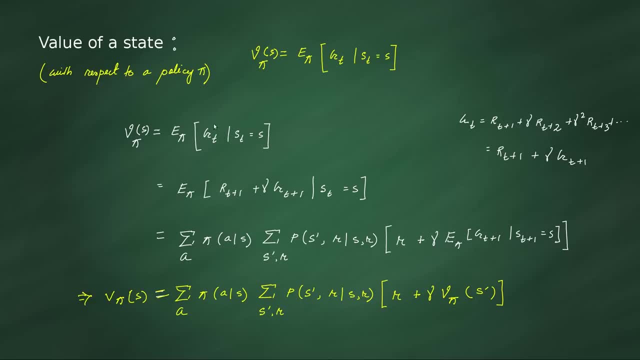 state. so you can see it's a expected uh total discounted reward and since it is gt, we can expand it like rt plus 1 plus gamma multiplied by gt plus 1. why we can do this, why how we can expand this value. just look at this equation. so it is gt plus rt plus 1 and we can proceed. 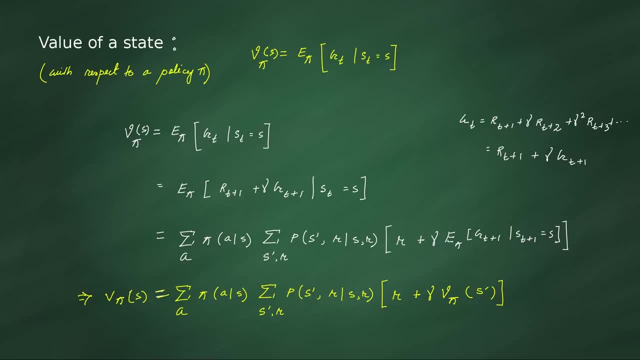 and you see what is the expected discounted reward and this is the value of the of the particular state. so you can see it's expected total discounted reward and since it is GT, we can expand it like RT plus 1 plus gamma multiplied by GT plus 1. why we can do this, why how we can expand this value, just look at this. 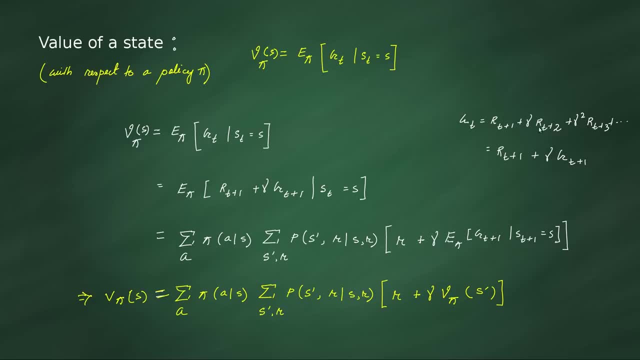 equation. so it is GT plus RT plus 1 and we can proceed like this and we can take this RT 1, T plus 1 as it is and we can add, we can add rest of the time, rest of the terms, by taking this discount factor as common, then we get a GT plus 1 inside. 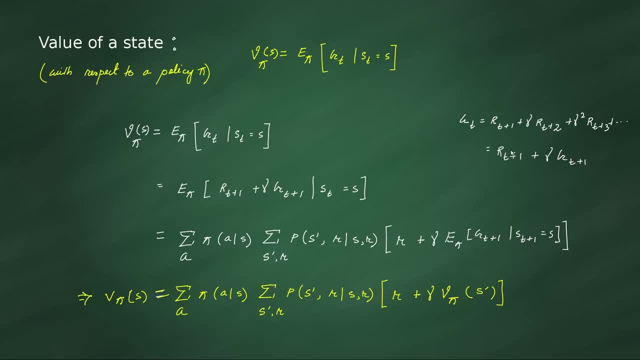 because it's the same expression inside, so we replace it and now it is expectation in the form of this expectation notation and we can expand it because we know the probability distribution. we assume that we know the probability distribution of actions for a particular state, which is the policy, and we know the transition dynamics of the 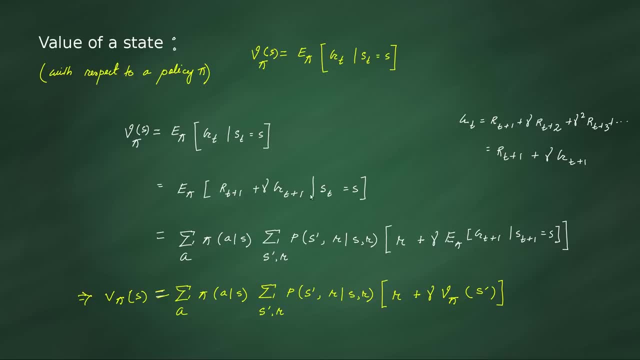 environment, so we can actually compute the expectation, like this properly, like with using probability distributions, and we get this equation and finally we have this expression for a value of a state like this. so you can see, here we are computing the value of a state using the value of the successive state. can you see that here? so this is the state where 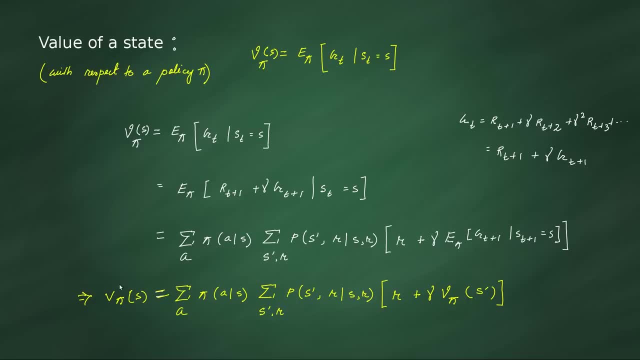 we are currently and we want to compute this state. so for that we can do like this and see- in this expression there is a term again- value of another state. this is the successive state. so this is like a recursive equation, because we can update the value of the current state. 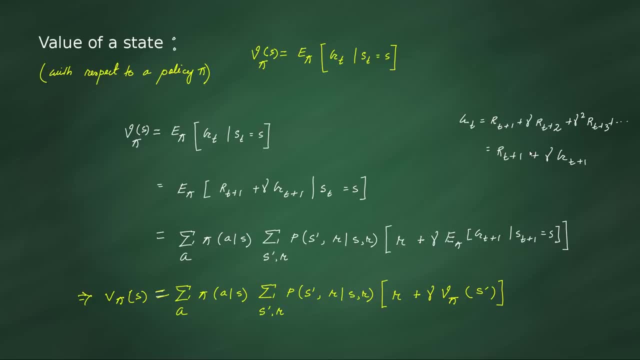 like this and we can take this rt 1, t plus 1 as it is and we can add, we can add rest of the time, rest of the terms, by taking this discount factor as common. then we get gt plus 1 inside, because it's the same expression inside, so we replace it and 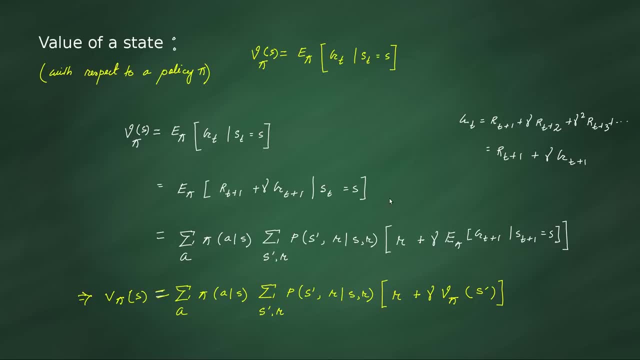 now it is expectation in the form of this expectation notation and we can expand it because we know the probability distribution. we assume that we know the probability distribution of actions for a particular state, which is the policy, and we know the transition dynamics of the environment, so we can actually compute the expectation like this properly, like 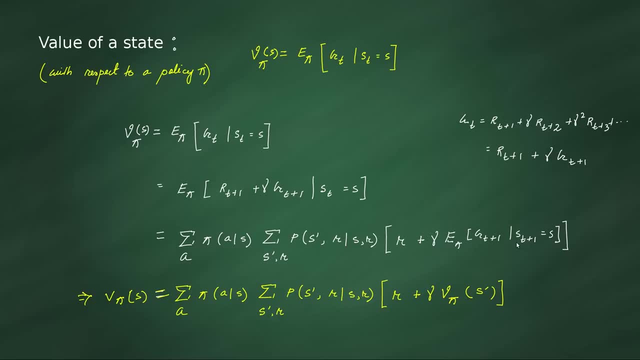 with using probability distribution. so we know the value of a particular stat to break it down into star and we don't need anyków to do that and we just set by our own calculations it's the value of the time that it is calculated and, of course, excellent. so here are the values of the state, like this, so you can see here we are computing the value of a state using the value of the successive state. can you see this here? so this is the state where we are currently and we want to compute this state. so for that we run on this. 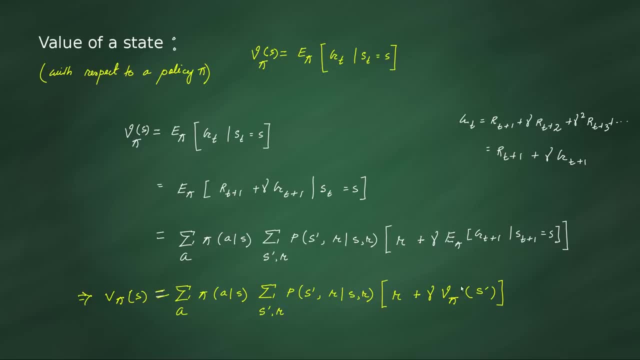 we can do like this and see in this expression there is a term again, value of another state, it is the successive state. so this is like a recursive equation, because we can update the value of the current state using the value of the successive state and we can also expand. 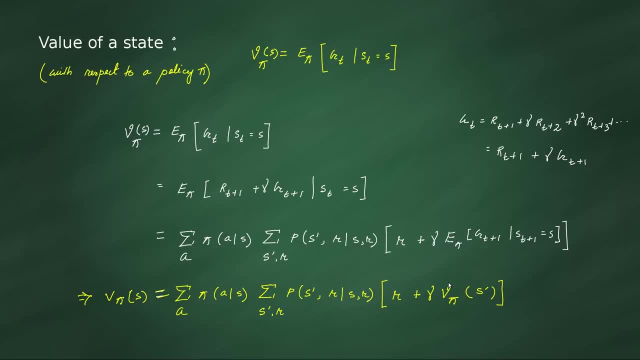 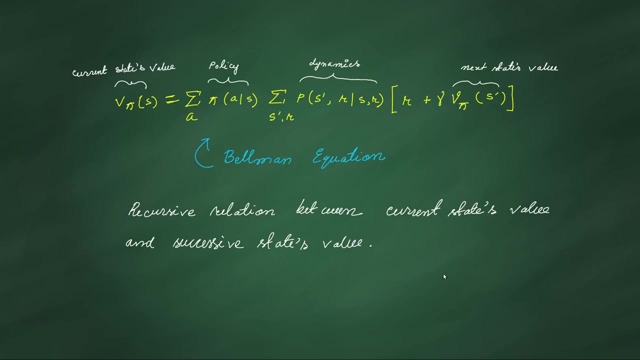 this using the whole equation. we can also expand this inside, inside the equation. so if we can expand this, expand this, expand this, then we will get a very huge equation. so yeah, so this is called Bellman equation. okay, so this is called Bellman equation. and here are 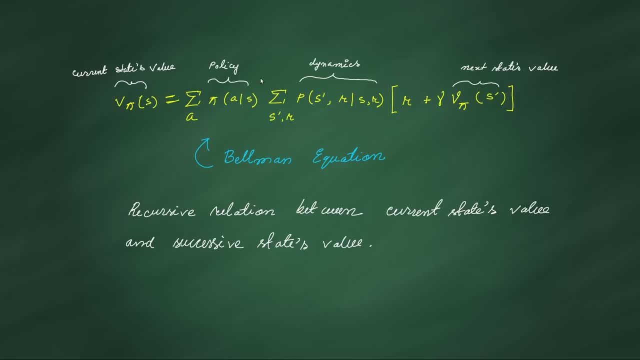 these terms I already mentioned. this is the current state, this is the policy, this is the dynamics and this is the next state's value. okay, so Bellman equation is very important and we will see Bellman optimally equation which we will use almost all the times in the upcoming classes. and let's go. 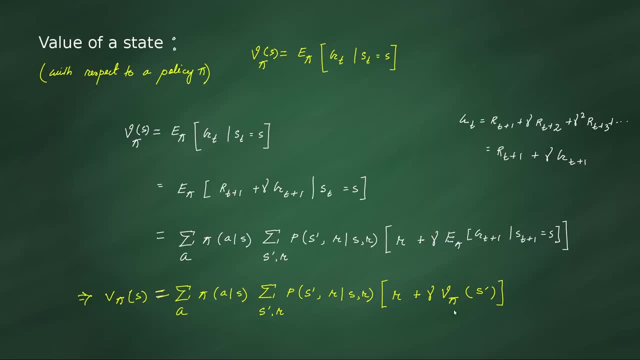 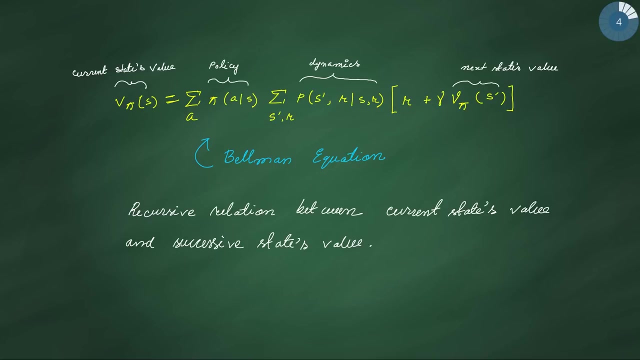 using the value of the successive state, and we can also expand this using the whole equation. we can also expand this inside, inside the equation. so if we can, if we expand this, expand this, expand this, then we will get a very huge equation. so yeah, so this is called Bellman equation, okay, so 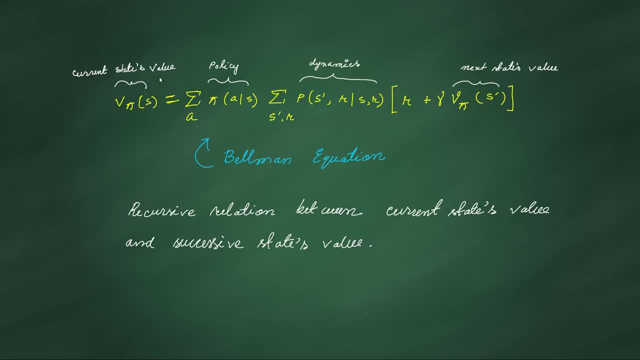 this is called Bellman equation and here are these terms I already mentioned: this is the current state, this is the policy, this is the dynamics and this is the next states value. okay, so Bellman equation is very important and we will see Bellman optimality equation, which we will use almost 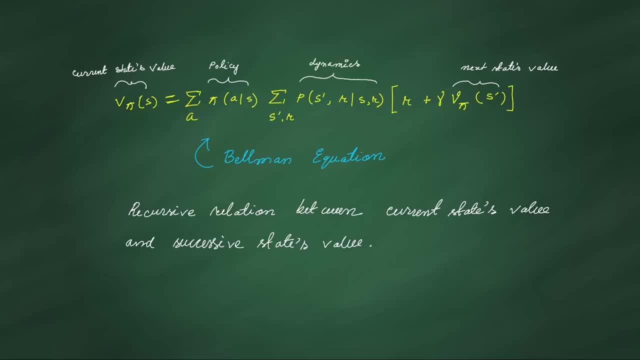 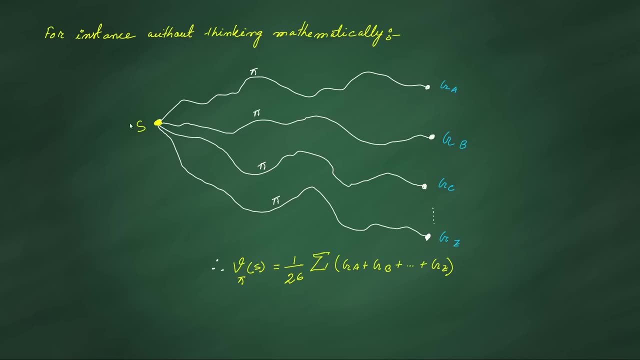 always all the times in the upcoming classes. and let's go to an example. what do we mean by value of a state in an intuitive way? so let's say you are in a particular state and you apply a policy, policy will tell which action to apply and you move to a different state and then in that state, 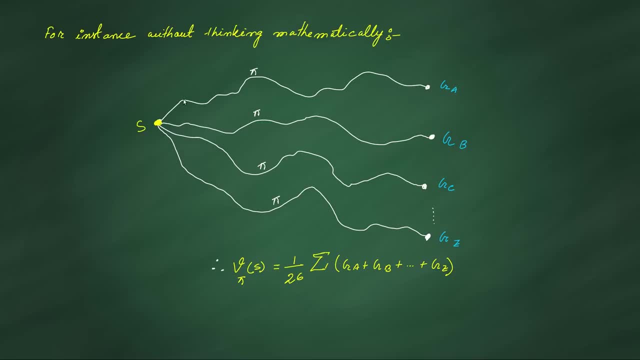 also policy will tell which action to take and then you apply next action. and in this way, suppose you move like this, since your environment is stochastic, like if you in a particular state, if you apply an action, you go to a different state, not the same state, all the time when you apply the same action. so what happens? 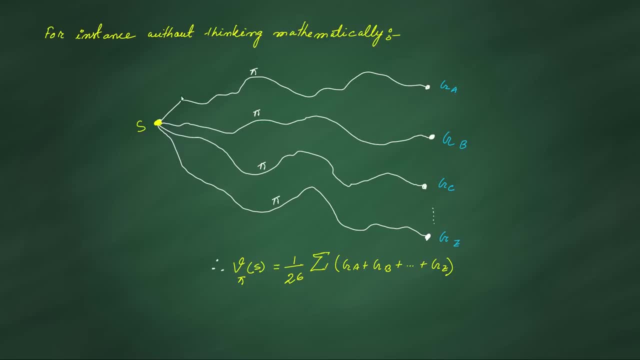 you'll take different trajectories, even if you are applying the same policy. you get different trajectory of different state trajectories, like this. so at the end of the trajectories, let's say you get a total discounted reward of reward of G a in this trajectory and GB in this trajectory and like this, and you 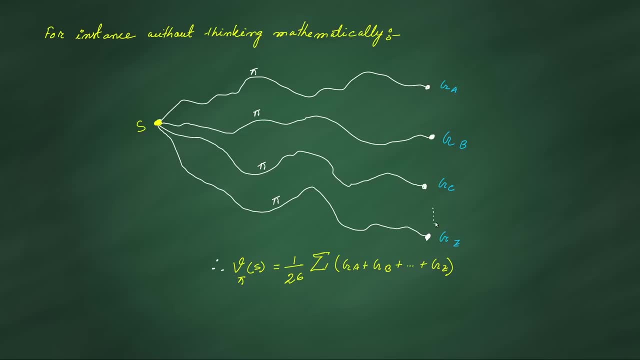 get enough for this trajectory. you get G, Z, so you have 26 total discounted reward now. so how do you calculate the value of a state? not, it's not called calculating, but it's like estimating the value of the state. so how will estimate the value of state? just, we take the average. right, we take the average like we had. 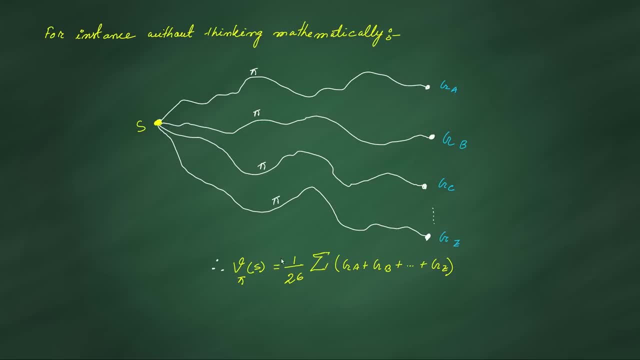 to an example. what do we mean by value of a state in an intuitive way? so let's say you are in a particular state and you apply a policy. policy will tell which action to apply and you move to a different state and then in that state also, policy will tell which. 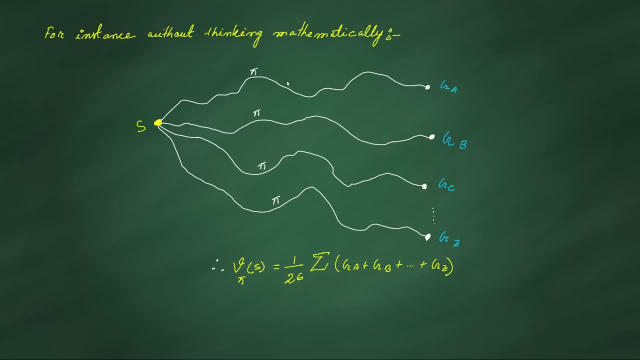 action to apply. so in this way, if you move from the Animation state and then you apply this action and then you define action and then you apply next action. and in this way, suppose you move like this, since your environment is stochastic, like if you in a particular state, if you apply an action, you go to a different state, not the same state. 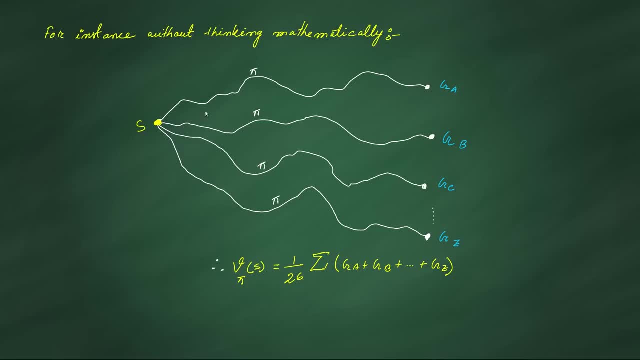 all the time when you apply the same action. so what happens? you'll take different trajectories, even if you are applying the same policy. you'll get different trajectory of different state, discounted reward of g, reward of ga in this trajectory and gb in this trajectory, and like this, and you get the in the for this trajectory, you get g, z, so you have 26 total discounted reward. 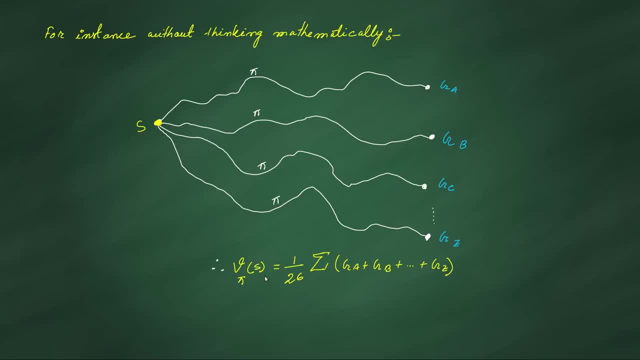 now. so how do you calculate the value of a state? i not, it's not called calculating, but it's like estimating the value of the state. so how will estimate the value of state? just, we take the average. right, we take the average, like we had 26 trajectories here and 26 total discounted. 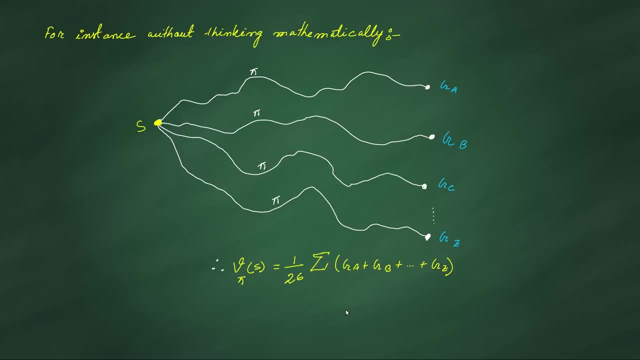 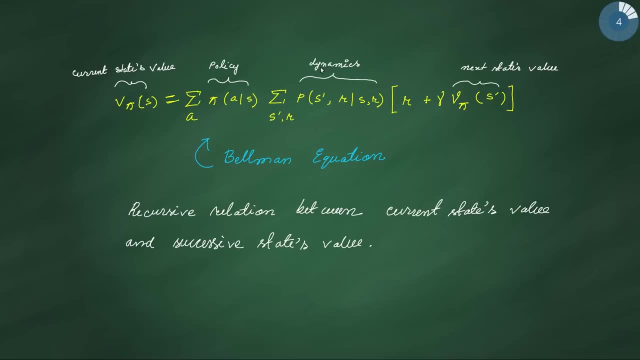 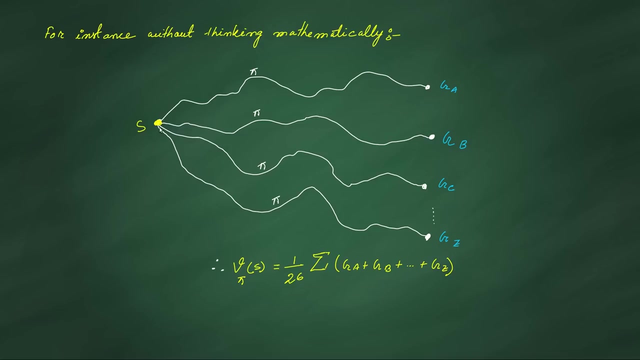 reward. so we'll add them and divide it by 26. so we have estimated the value of the state. but in the previous equation we are not actually estimating. we are actually calculating the value of the state using the probability distribution. but this is the kind of rough estimation of the value of the state, just to be intuitive, to get the intuition. 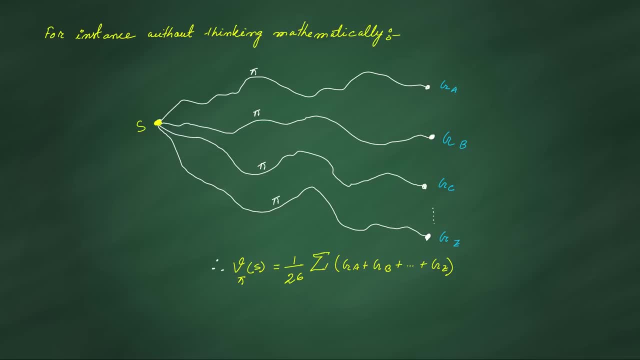 behind what is the value of a state. so it is just kind of average of all the possible total discounted reward you can get using a particular policy. and since your environment is stochastic, you get different total discounted reward every time you apply the same policy but your. but if your environment is not stochastic, if you apply the same policy, if you get the same, 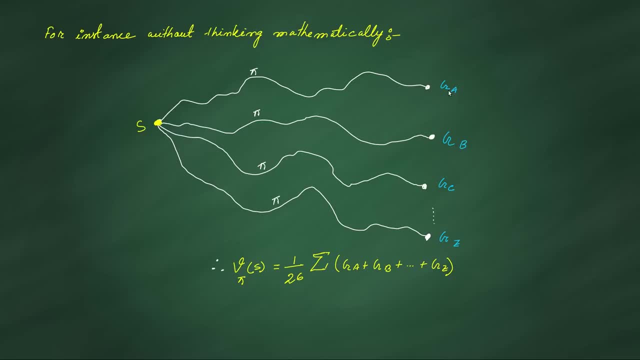 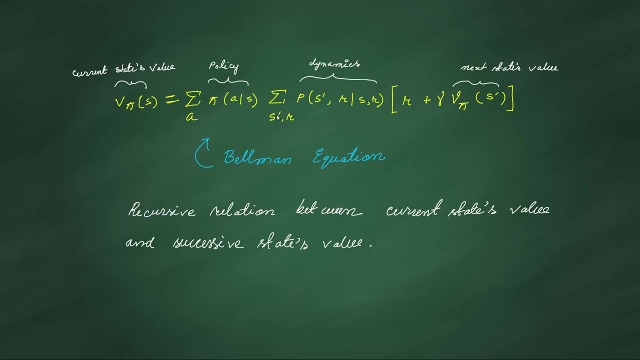 twenty, twenty-five, six trajectories here and twenty-six total discounted reward. so we'll add them and divide it by 26. so we have estimated the value of the state. but in the previous equation we are not actually estimating. we are actually calculating the value of the state using the probability distribution. but this is 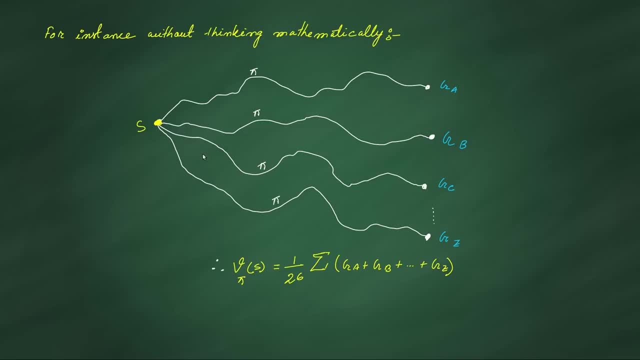 the kind of rough estimation of the value of the state, just to be intuitive, to get the intuition behind what is the value of a state. so it is just kind of average of all the possible total discounted reward you can get using a particular policy. and since your environment is stochastic, you get. 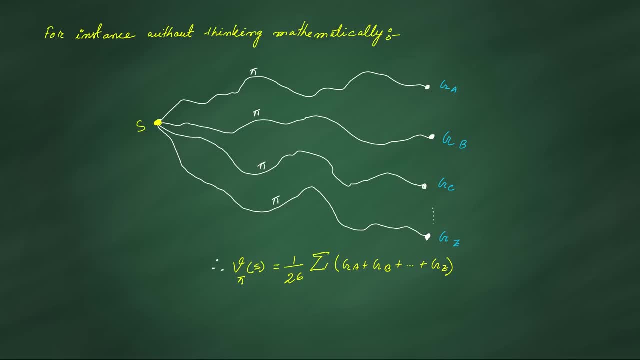 different total discounted reward every time. you apply the same policy but your. but if your environment is not stochastic, if you apply the same policy, if you get the same trajectory all the time, then your value is just the same. it's the same the single total discounted reward, because you get the 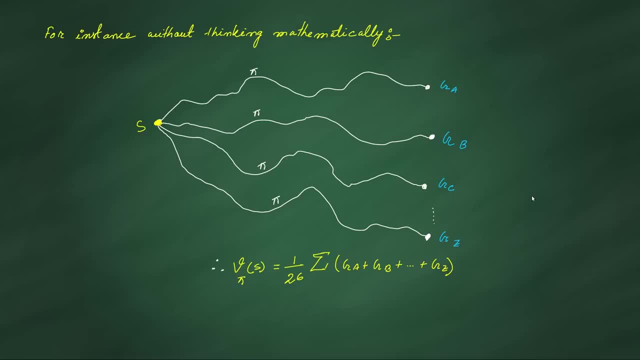 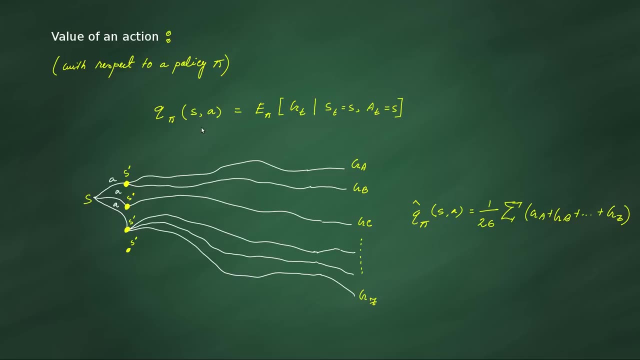 same trajectory all the time, if your environment is not stochastic. so we can also define a value of an action. so what is the value of an action? so, in a particular state, if you apply an action and then onwards, if you apply a policy for a particular time steps, then whatever total discounted reward. 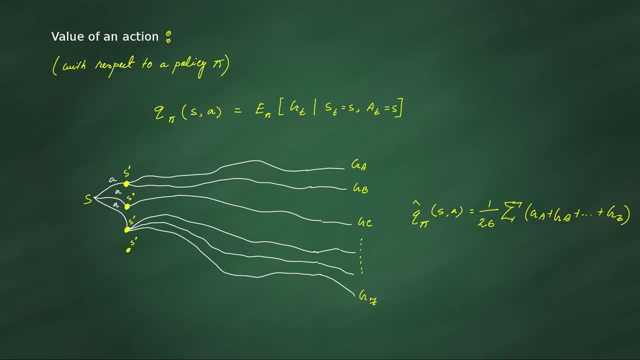 expected total discounted reward you receive. it's called the value of the value of an action. that means for a particular state, you have to first apply an action, the action for which you are going to estimate the value. so, for a particular state, you first apply an action and then after, after applying the 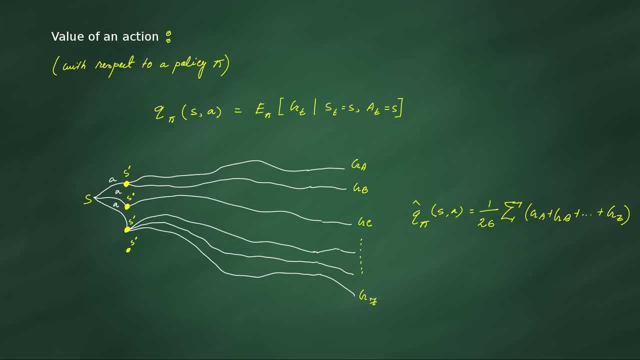 action. you go to a different state and then onwards, you apply the particular policy. okay, you apply a particular policy and you get different trajectories from different states. like this: you apply the same action from state s. you ended up in this state, sometimes in these states, because, again, I told you, 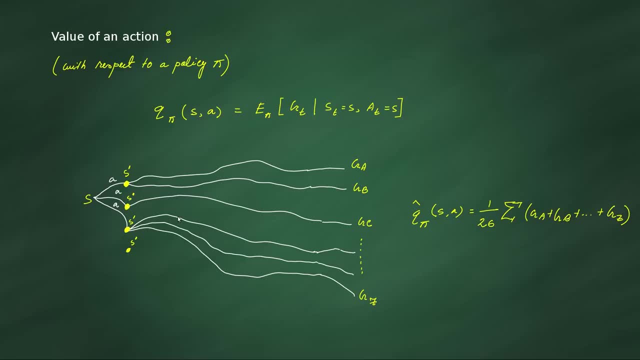 it's a stochastic environment. you will never go to the same state again and again. so, and then onwards you apply the fixed policy for the policy for which you are computing the action value, and then you sum all the total discounted reward and then you take the average. then it's called the estimation of value of an. 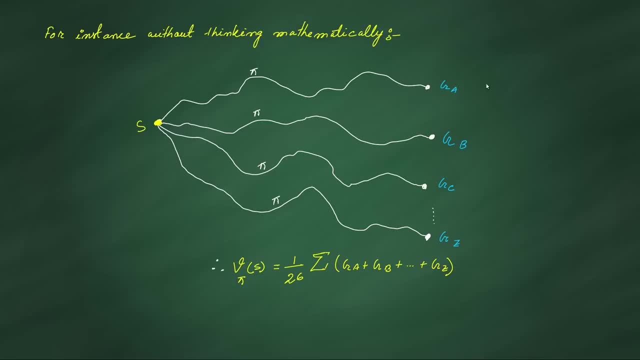 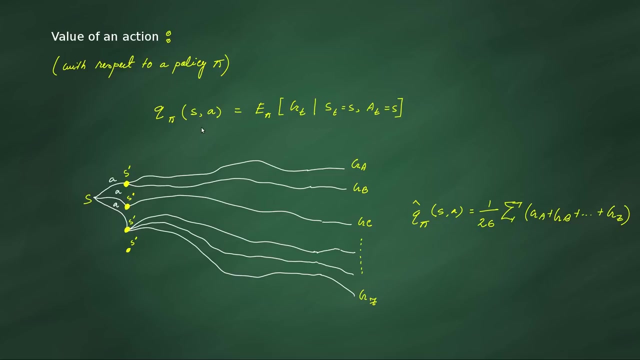 trajectory all the time, then your value is just the same. it's the same, the single total discounted reward, because you get the same trajectory all the time, if your environment is not stochastic. so we can also define a value of an action. so what is the value of an action? so, in a particular state, if you apply an action, and then onwards, if you apply, 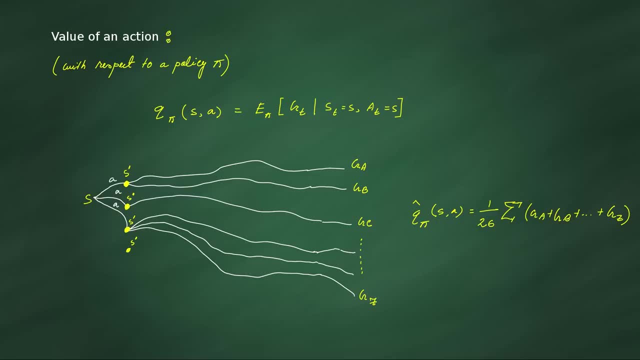 a policy for a particular time steps, then whatever total discounted reward you receive, it's called the value of an action. that means for a particular state, you have to first apply an action, the action for which you are going to estimate the value. so, for a particular state, you first apply an action and then, after after applying the action, you go to a different. 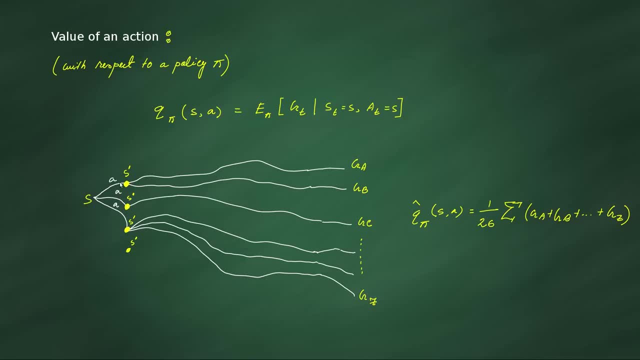 state and then onwards, you apply the particular policy. okay, you apply a particular policy and you get different trajectories from different states. like this: you apply the same action from state as you ended up in this state. sometimes in this stage- because, again I told you, it's a stochastic environment- you will never go to the same state again and again. so 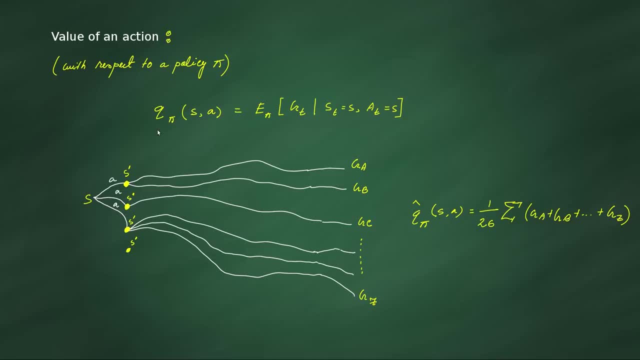 and then onwards you apply the fixed policy for the policy for which you are computing the action value and then you sum all the total discounted reward and then you take the average. then it's called the estimation of value of an action. but you can also compute this value in closed form, like previous. 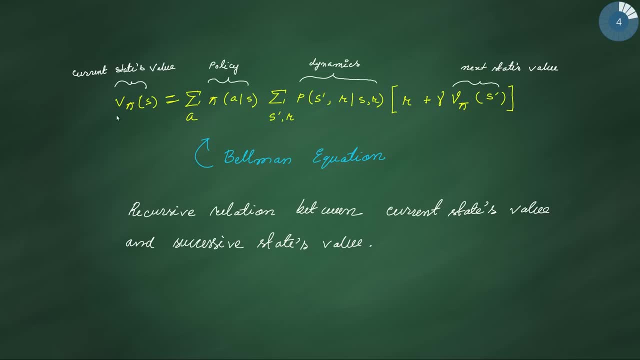 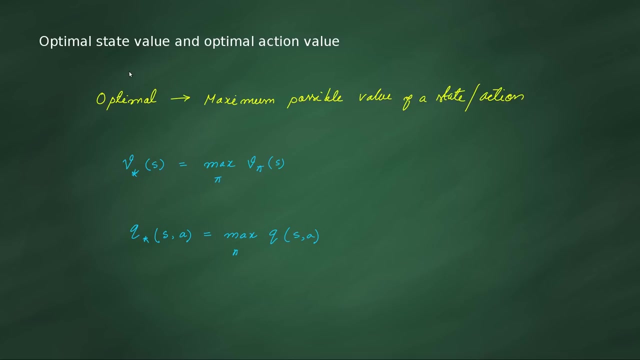 expression like, like this expression, as you know, the probability of probability, transition, probability of the environment and policy. so you can compute this value in the cool flow, in a closed form. now let's say what is optimal state value and optimal action value of a particular state. so for a 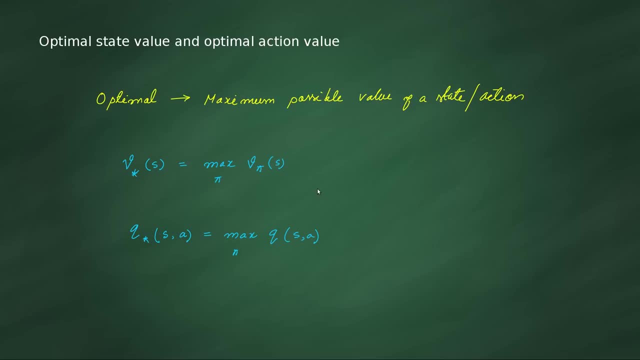 particular state. the optimal state value is the maximum state value. if your goal is to maximize the reward, then in the environment, then is the maximum possible action value for a particular state, or maximum possible state value for a particular state is the optimal. so when you get this optimal value, when you 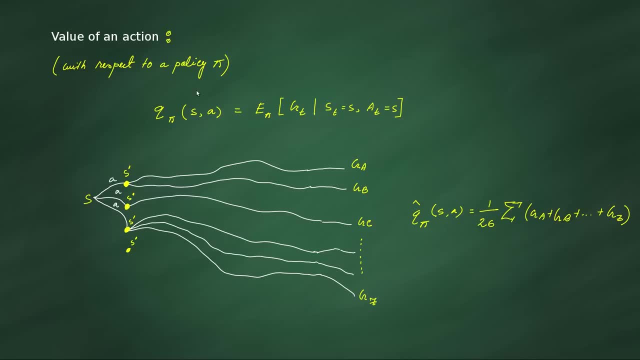 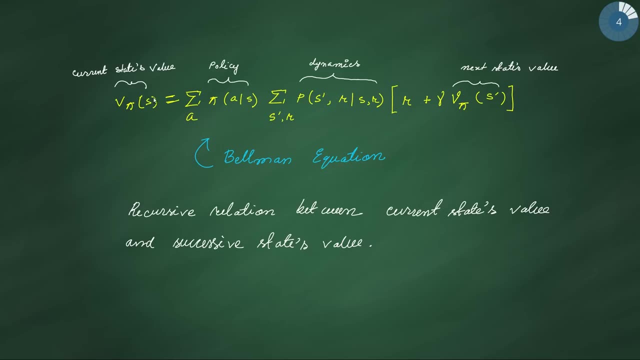 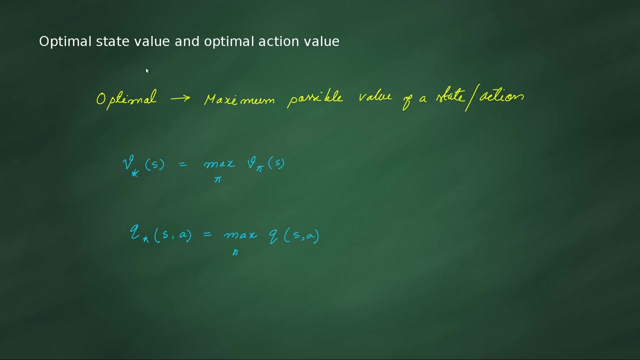 action. but you can also compute this value in closed form, like previous expression, like, like this expression, as you know, the probability of probability, transition, probability of the environment and the policy. so you can compute this value in a closed form. now let's see what is optimal state value and optimal action. value of a. 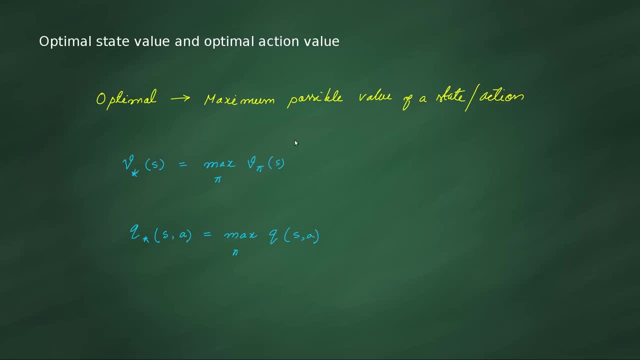 particular state. so for a particular state, the optimal state value is the maximum state value. if your goal is to maximize the reward, then in the environment, then is the maximum possible action value for a particular state or maximum possible state value for a particular state. it's the optimal. so when you get this optimal, 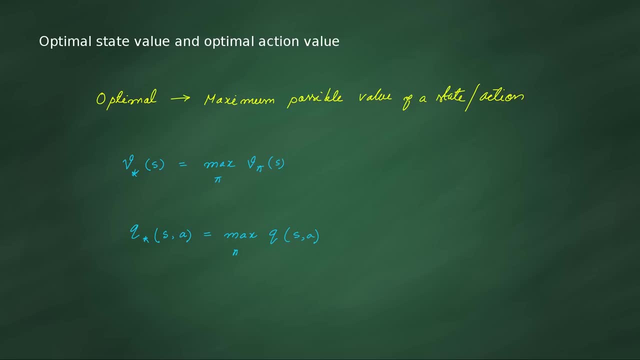 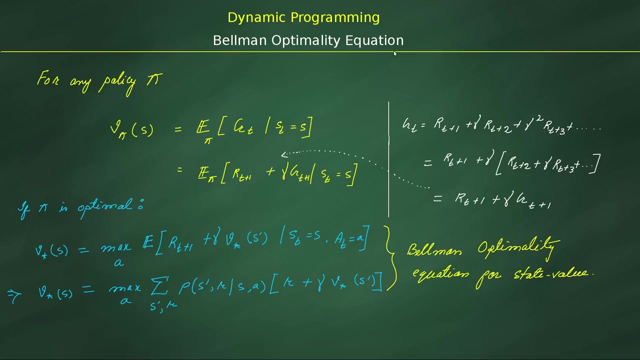 value when you have an optimal policy. optimal policy means the best policy, the policy that gives you the best reward, and similarly, the same case for optimal action value. so let's look at the element optimality equation. so, as we have seen this equation previously, the value of a particular state with respect to an, but to a with. 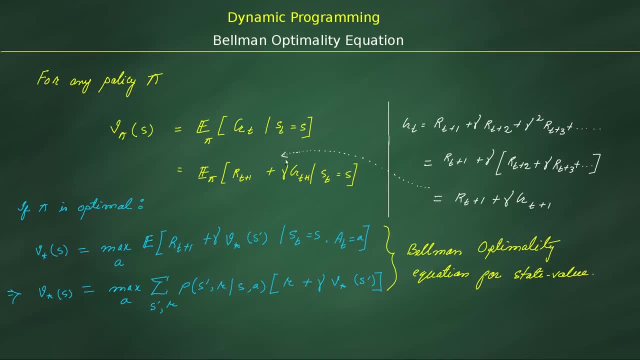 respect to a policy. we expand this like this- we talked about this before- then. if our policy is optimal, if we take the optimal policy, then what will happen? we can replace this thing like this: we can get half of this one among the� JUNE- the number of tasks as an element. 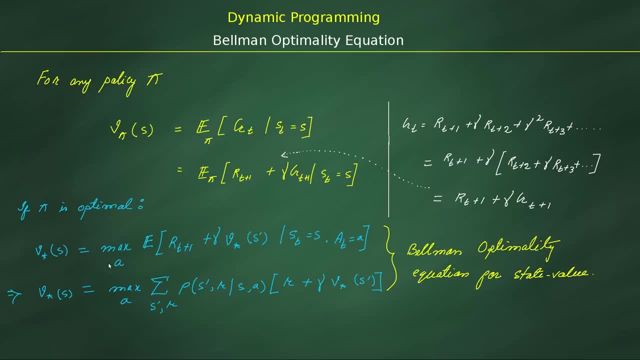 okay, we are going to divide theorem- which we are doing, the value error equation on theåtter equation, which I told you. we divide the value as a probability of serious action. well, if you take the 100 percent casebai in the as the very maximum, 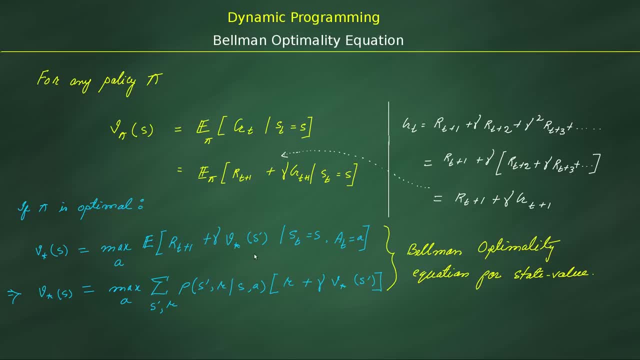 value of a second action values. the values which had higherbildt with respect to force stay equal plus discounted optimal value for the successive state. uh, expectation of this term- actually, not this exact value, but expectation of this term, and this is called bellman optimality equation. and 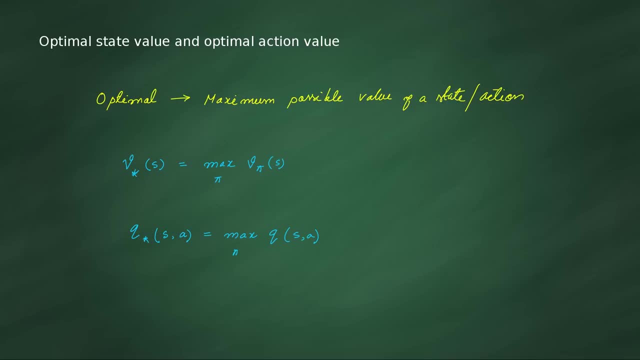 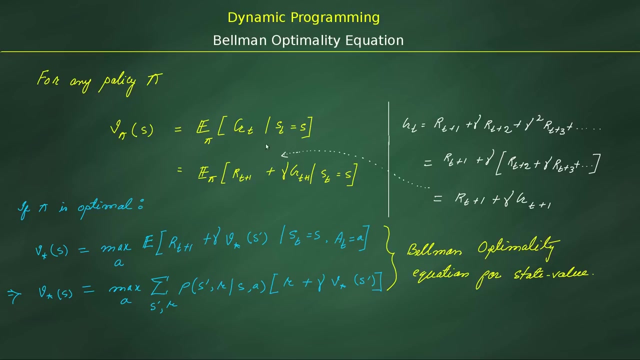 have optimal policy. optimal policy means the best policy, the policy that gives you the best reward, and similarly, the same case for optimal action value. now let's come to Bellman optimality equation. so, as we have seen this equation previously, the value of a particular state with 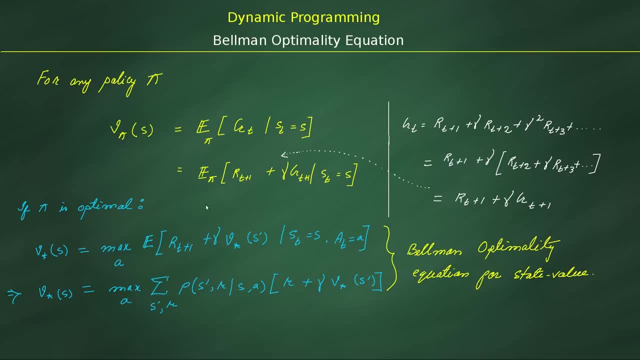 respect to an, but with respect to a policy. we expand this like this. we talked about this before then: if our policy is optimal, if we take the optimal policy, then what will happen? so we have this option. we can replace this thing like this: we then value of a. 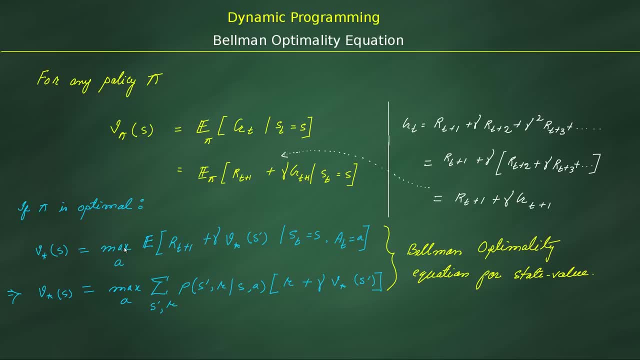 state, then the optimal value of a state will be the same as applying the action that maximize this expected term. okay, it's RT plus one next reward and then discounted optimal state value for the next state. are you getting? it's a slightly complicated thing, so it's like the optimal value for a state will be a. 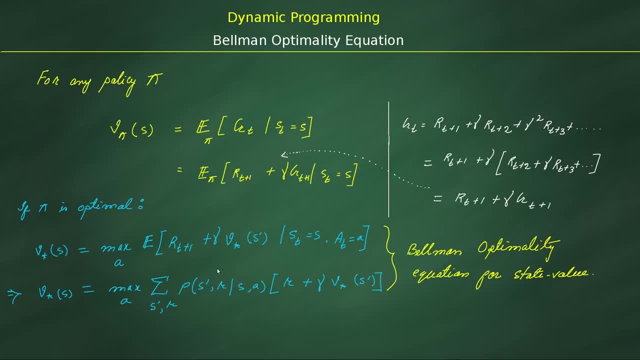 state equal to the sum of the reward plus discounted optimal value for the successive state, expectation of this term. actually, not this exact value, but expectation of this term, and this is called Bellman optimality equation, and we will be using this equation quite often in our next videos. and then, since 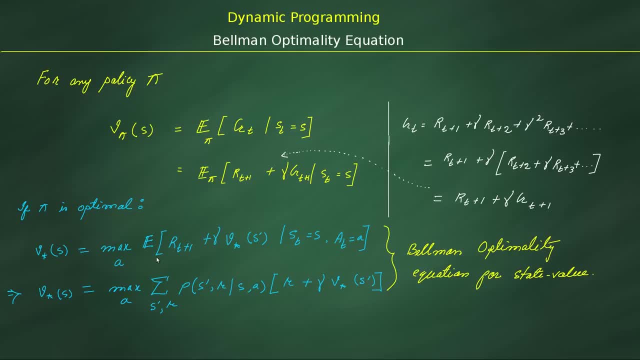 again, this is expectation and we know the probability distribution of the environment. we can simply expand it like this for a for for an action that maximize this term, and we can simply expand it like this. you can refer to the previous slides actually how we have expanded this term and this is called the bellman optimality equation. we also have this. 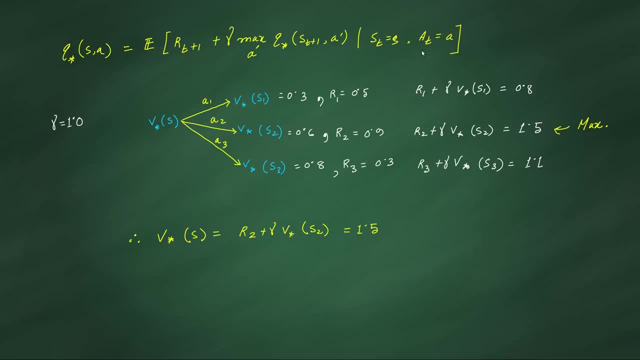 bellman, optimality for the action value. it's the same thing, it's almost similar. let's take an example, because in terms of equation it's always difficult to understand. so let's take an example. suppose we have to estimate the optimal value for this particular state. so what we will do, we'll. 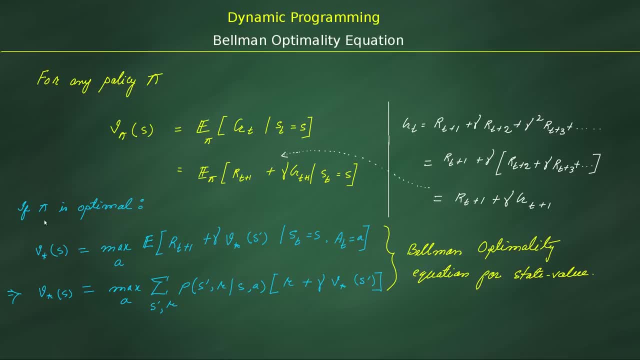 we will be using this equation quite often in our next videos. and then, since again, this is expectation and we know the probability distribution of the environment, so we can simply expand it like this for a for for an action that maximize this term. and we can simply expand it like this- you can refer to the previous slides- actually how we 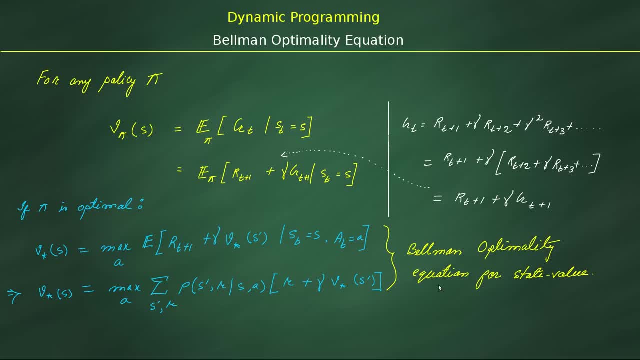 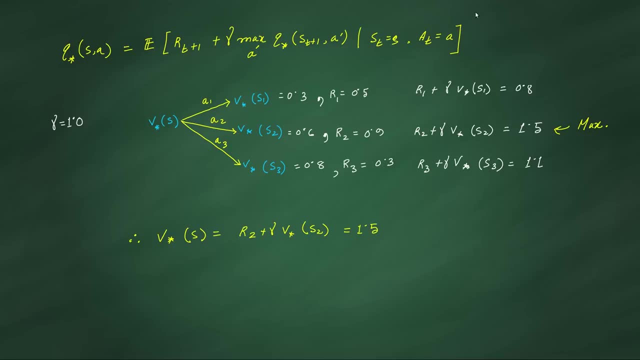 have expanded this term and this is called the bellman optimality equation. we also have this bellman optimality for the action value. it's the same thing, it's almost similar. let's take an example, because in terms of equation it's always difficult to understand. 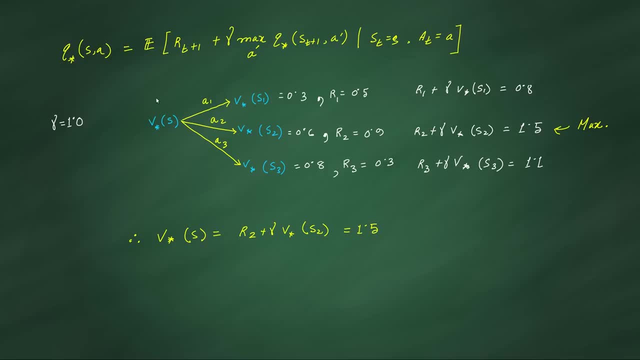 so let's second example: suppose we have to estimate the optimal value for this particular state. so what we will do, we'll apply all the actions first. okay, so we are estimating right, so we'll apply all the actions. let's say, after applying action a1 we end up at the state s1, and if we apply action a2, then 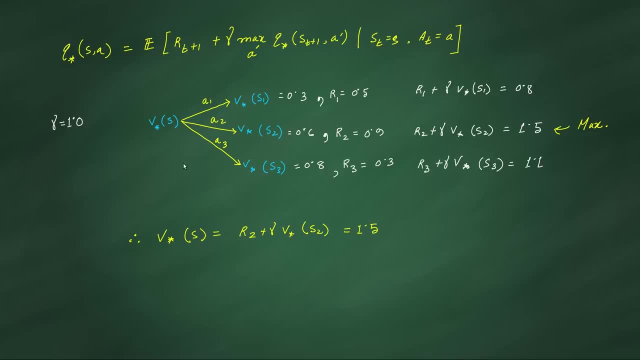 we end up at action state s2 and similarly in s3 if we apply action a3. so let's say the optimal state value for state 1 is 0.3 and for this it's 0.6 and for this it's 0.8. okay. and also we say: 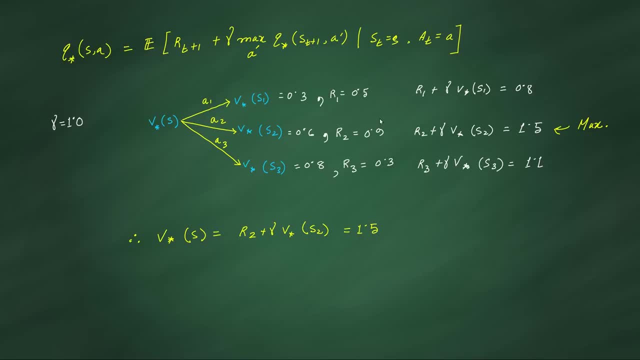 that in this state you get reward 0.5 and here it's 0.9 and in this state is 0.3. so what we have done is we have applied action a1 and we end up at action s2 and similarly in s3, if we apply. 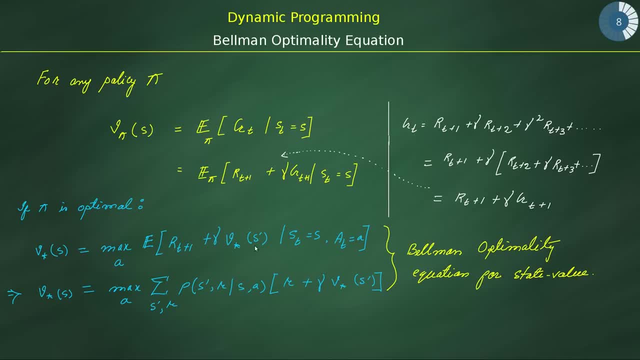 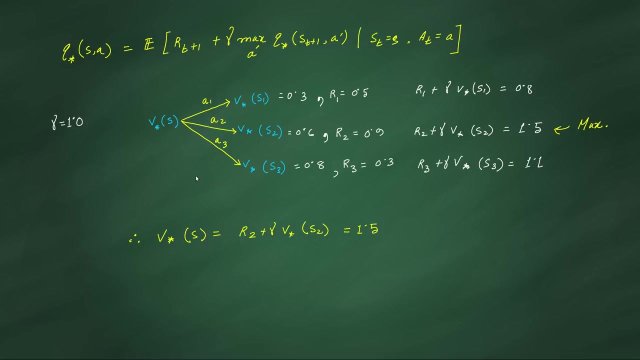 action a1, we have to see, we have to maximize this term right, this term, the expectation of this term, rt plus one, the reward of the next state, then discounted optimal value of the next state. so since we are talking about here in this example, it's deterministic. so if we apply action a1, we 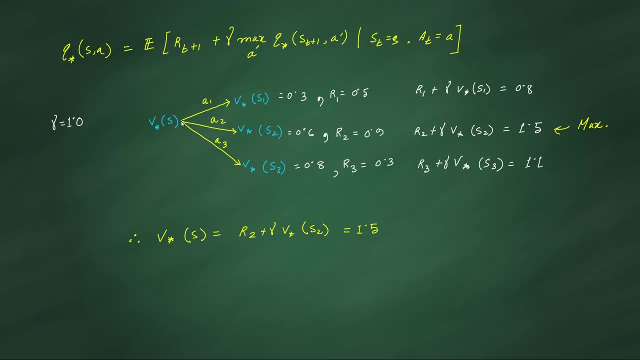 apply all the actions first. okay, so we are estimating right, so we'll apply all the actions. let's say, after applying action a1, we end up at the state s1, and if we apply action a2, then we end up at action state s2 and similarly. 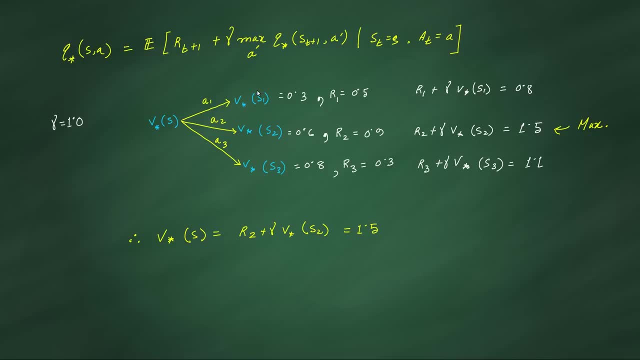 in s3, if we apply action a3. so let's say the optimal state value for state 1 is 0.3 and for this it's 0.6 and for this it's 0.8. okay, and also we say that in this state you get reward 0.5 and 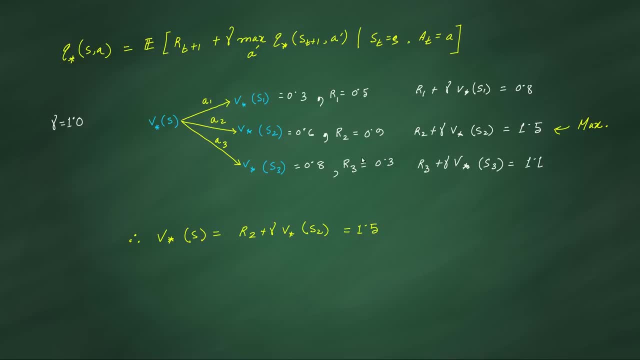 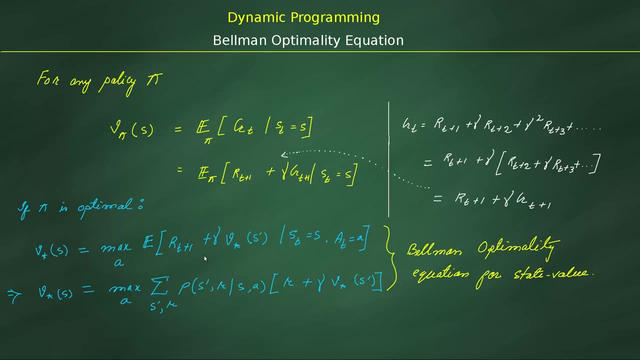 here it's 0.9 and in this state is 0.3. so what we have to see, we have to maximize this term right, this term. the expectation of this term, rt plus 1, the reward of the next state, then discounted optimal value of. 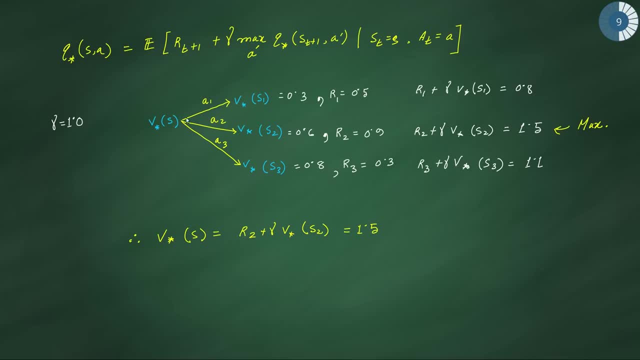 the next state. so since we are talking about here in this example, it's deterministic. so if we apply action a1, we directly go, always go, to state s1. so it's deterministic. so we don't have to take the expectation, we just have to add the values r1, the next reward plus discounted. we assume the. 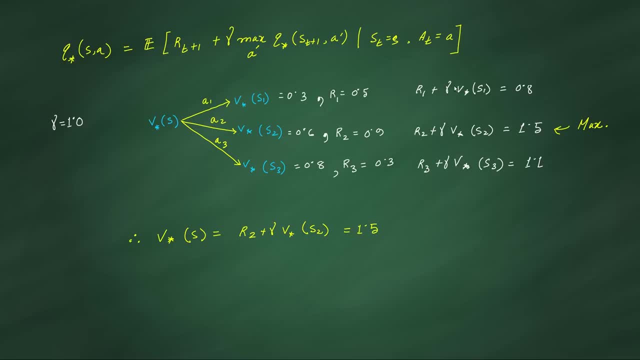 discount fator is 1 here, so we multiply it with the optimal state value for this particular state and we get 0.8 here, and for the second case we get 1.5, and in the third case we get 1.1. so what is the? 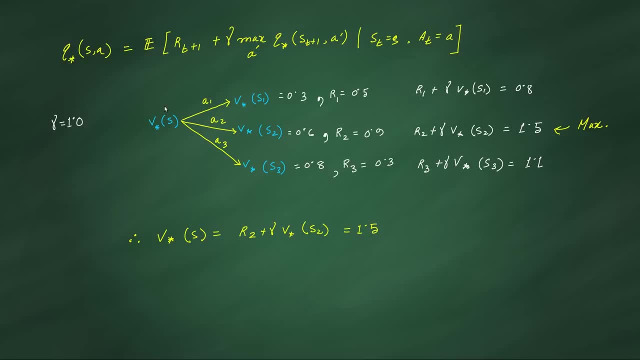 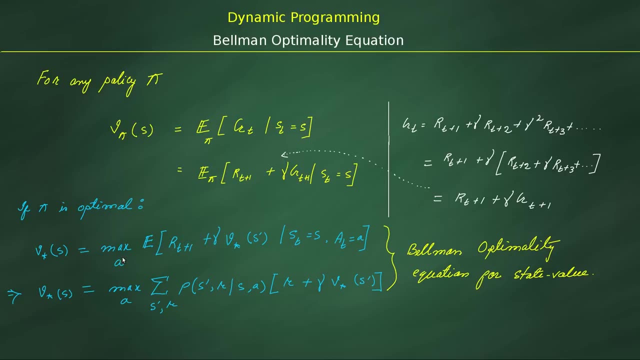 optimal value for this state. so it is the maximum. so you remember, we are maximizing, right, we are maximizing 0.1 with action. so we take different actions and we see the action that maximizes this and we take the maximum value. and the maximum value of this is the. 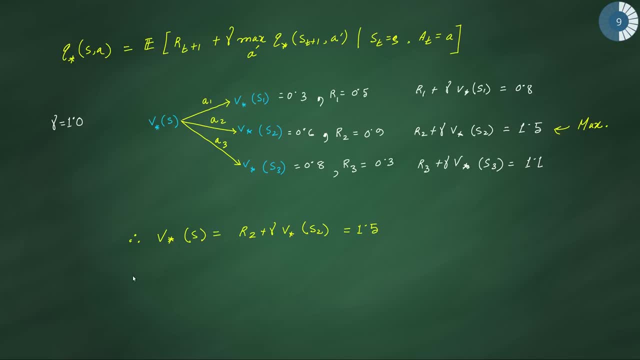 optimal value for the state. so here also, we took the maximum, we took different actions here and we added the term- we don't have to take the expectation here, because we are dealing with deterministic environment in this particular example- and we took the maximum here, and and this is the value- 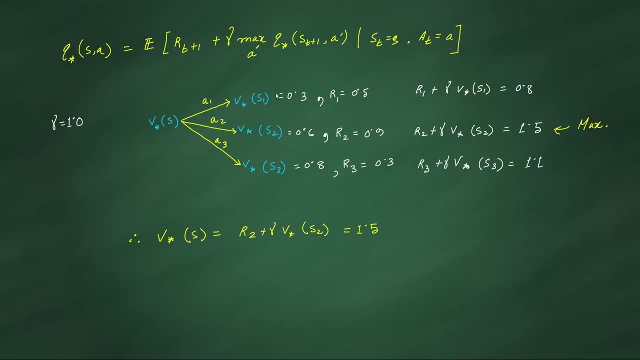 always go to state s1, so it's deterministic. so we don't have to take the expectation, we just have to add the values r1, the next reward, plus discounted. we assume the discount factor is one here, so we multiply it with the optimal state value for this particular state and we get. we get 0.8 here. and for the second case, 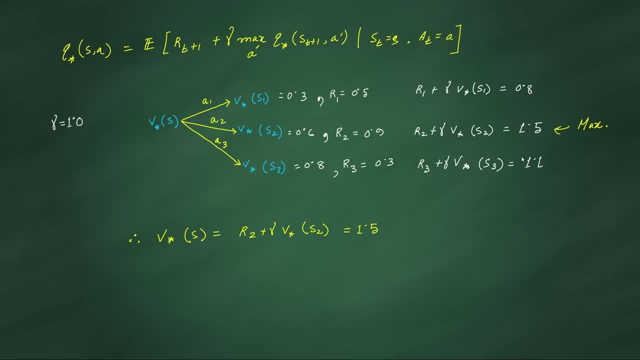 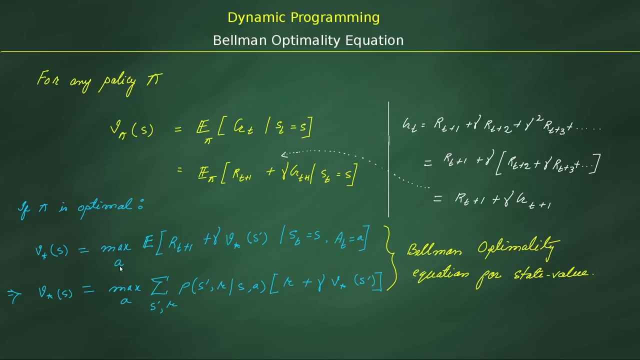 we get 1.5 and in the third case we get 1.1. so what is the optimal value for this state? so it is the maximum. so remember, we are maximizing, right, we are maximizing with action. so we take different actions and we see the the action that maximizes this and we take the maximum value and the maximum. 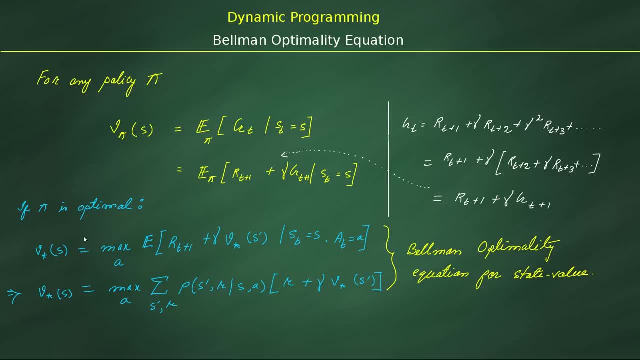 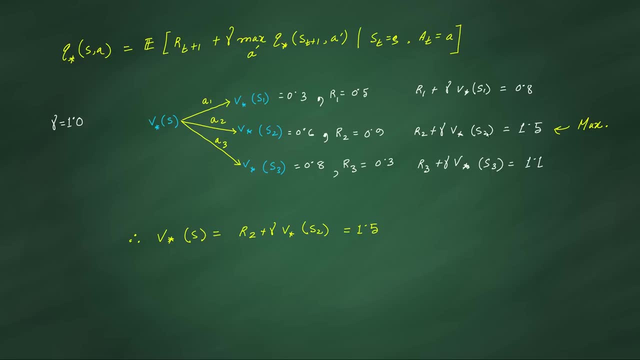 value of this is the optimal value for the state. so here also we took the maximum, we took different actions here and we added the term- we don't have to take the expectation here, because we are dealing with deterministic environment in this particular example- and we took the maximum here and- and this is the value of the state- 1.5. now. 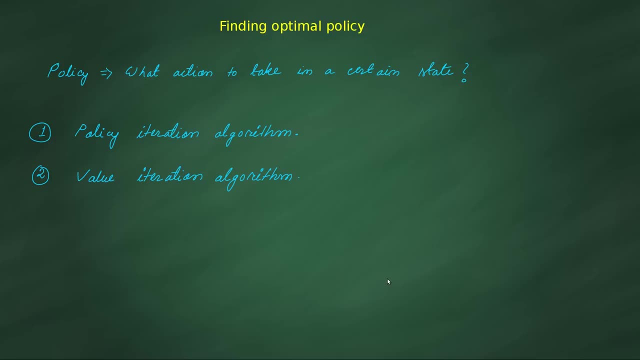 the question is how to find optimal policy. that means what action to take in a certain state to maximize the reward, the total discounted reward. so for this, who will now talk about two algorithms, one is called policy iteration algorithm and the second one is value iteration algorithm- policy. 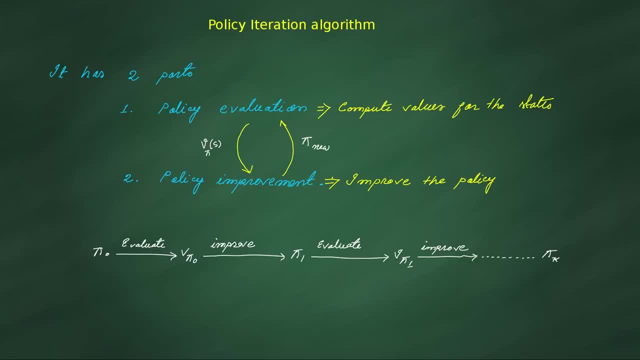 algorithm actually has two parts. the first one is policy evaluation. the policy evaluation: it computes values, state values for all the states in the environment using the policy, and this policy is provided by policy improvement process. so this part provides the policy and it computes the state value for all. 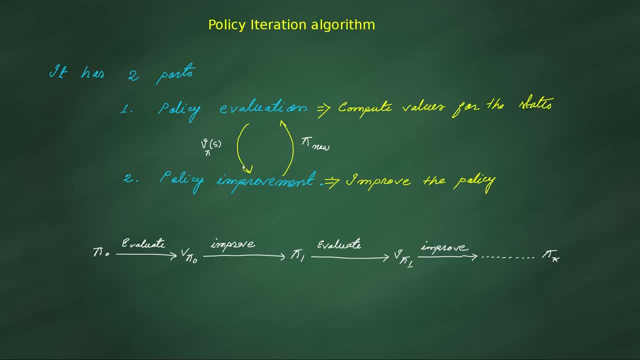 the states and it gives the state values to the policy. and looking into the state values evaluated by the policy evaluation part, the policy improvement part improves the policy so that it can get better state values. better means higher state values, so it proceeds like this. so first we have to set a random 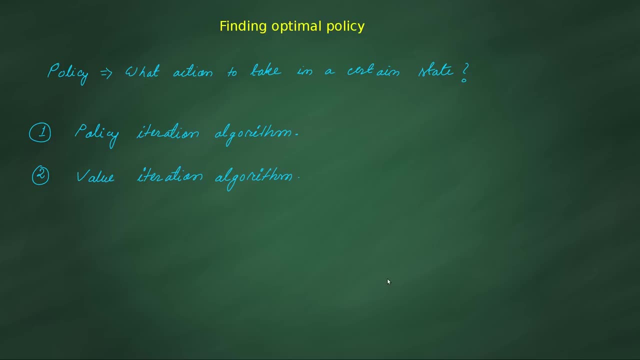 of the state 1.5. now the question is how to find optimal policy. that means what action to take in a certain state to maximize the reward, the total discounted reward. so for this we'll now talk about two algorithms. one is called policy iteration algorithm and the second one is value iteration algorithm- policy. 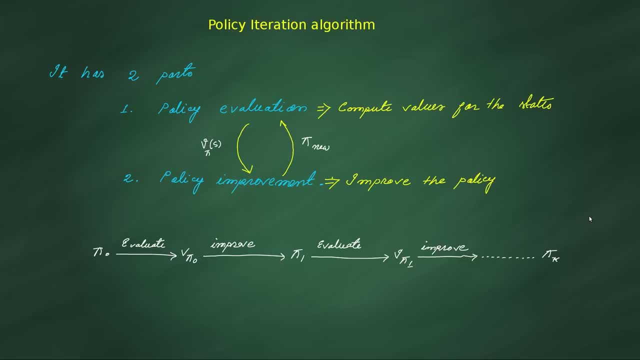 iteration algorithm actually has two parts. the first one is policy evaluation. yet the policy evaluation? it computes values, state values for all the states in the environment using the policy, and this policy is provided by policy improvement process. so this part provides the policy and it computes the state value for all. 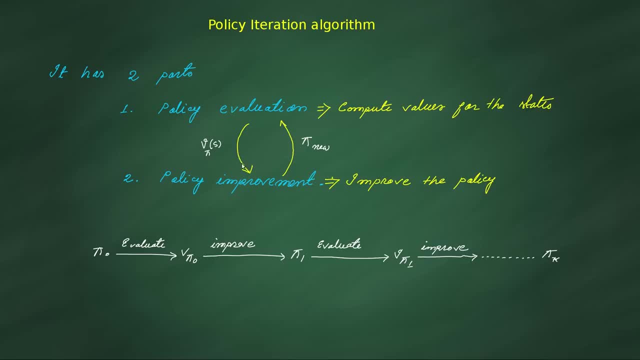 the states and it gives the state values to the policy. and looking into the state values evaluated by the policy evaluation part, the policy improvement part improves the policy so that it can get better state values. better means higher state values, so it proceeds like this. so first we have to set a random policy. 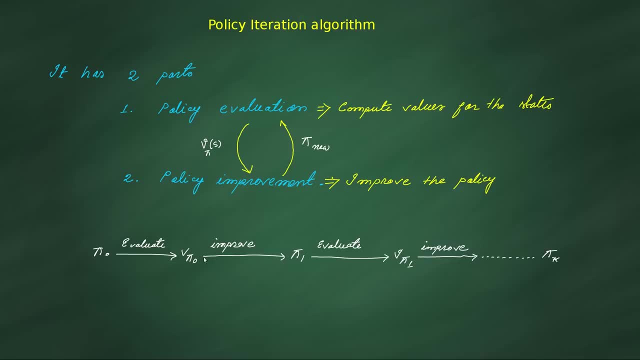 then policy evaluation will evaluate the value functions like state values for that particular policy. then policy improvement part will improve the policy and we get policy pi 1. and then policy evaluation will evaluate the policy to compute the state values and from the state values the policy improvement part improves the policy until we get the optimal policy and here algorithm. 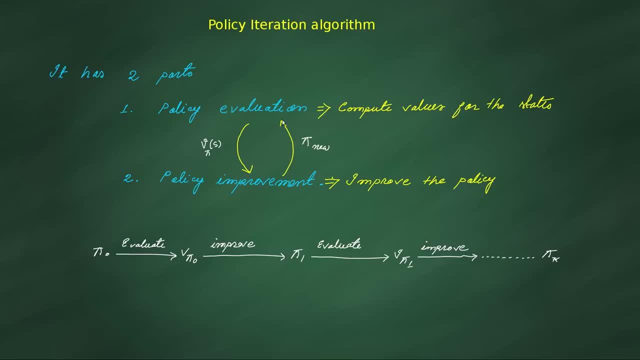 stops. so it's like communicating, like back and forth. it gives the policy, it gives back computed values and looking at the computed values, it again improves the policy and it like running a loop until we get the optimal policy. so let's see the algorithm in detail, so like individual parts first. so this is the iterative policy evaluation. so policy. 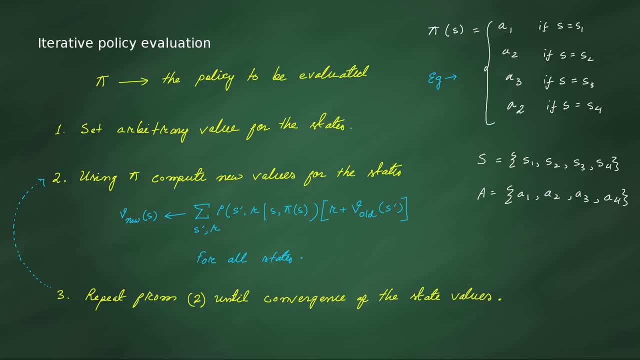 evaluation part is actually iterative. policy evaluation is also a loop actually. so how it is done, so first we we get the policy from the policy evaluation part and then we get the policy improvement part. right, if you are first starting the algorithm, then this policy will be a random. 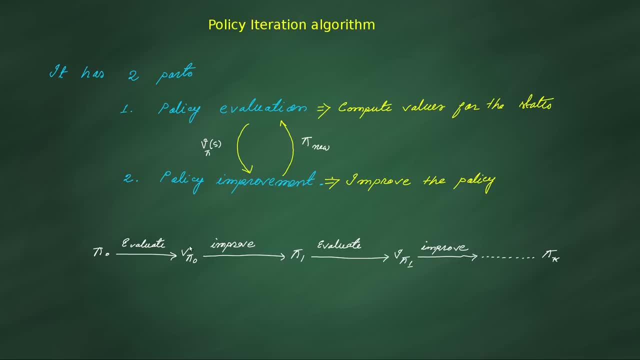 policy, then policy evaluation will evaluate the value functions like state values for that particular policy, then policy improvement part will improve the policy and we get policy pi 1. and then policy evaluation will evaluate the policy to compute the state values and from the state values the policy improvement part improves the policy until we get the 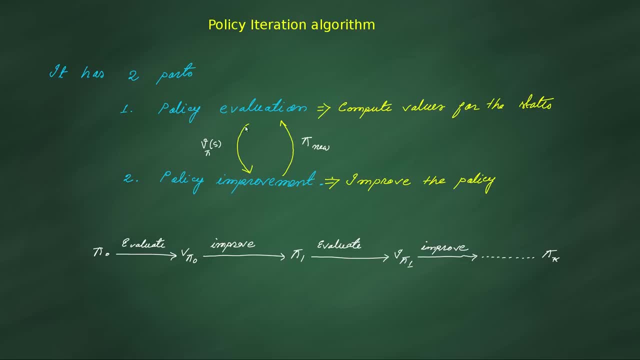 optimal policy and here algorithm stops. so it's like communicating, like back and forth. it gives the policy, it gives back computed values and looking at the computed values, it again improves the policy and it like running a loop until we get the optimal policy. so let's see the algorithm in 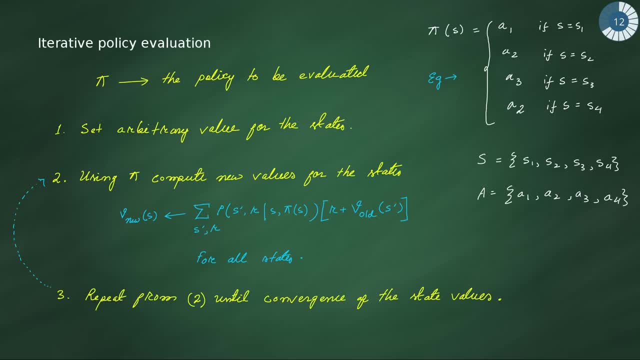 detail. so like individual parts first. so this is the iterative policy evaluation. so policy evaluation part is actually iterative. policy evaluation is also a loop actually. so how it is done. so first we, we get the policy from the policy improvement part right, if you are first starting the algorithm, then this policy will be a random policy. so when i say it's a 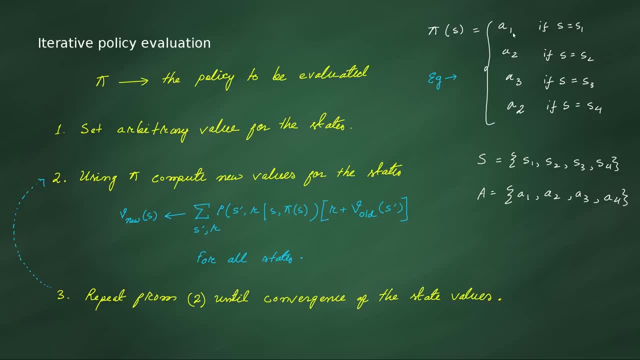 policy. it's just a table, like for a particular state. if your state is s1, then you apply action a1. if your state is a2, s2, then you apply a2. so it's like a table. so you randomly initialize this table. you can set like zero, zero, zero, zero, zero action, or just left, left, left, left, left, action. 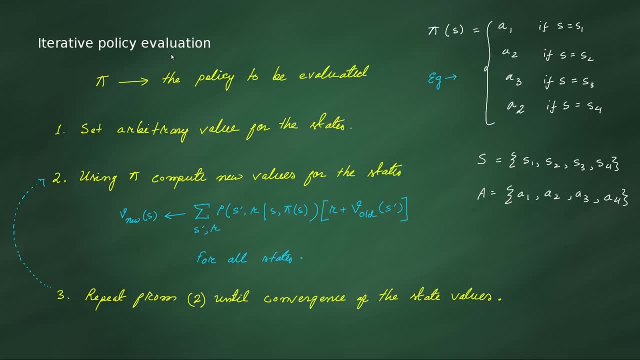 initially, and then this policy evaluation part evaluate the values for all the states. so it evaluates the values for all the states. you remember this is the equation for value function computation, the value value computation. so this is the equation you remember. so it takes the old value of the states. old values are also like randomly initialized set, arbitrary set, arbitrary. 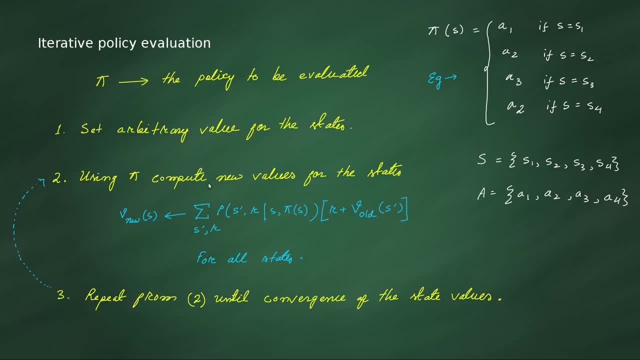 value for the states and using pi, compute new values for the states. so first you have to set the arbitrary states, also for the, for the environment. so we take, we can take zero, zero, zero everywhere, or we can take one, one, one, one, one everywhere. whatever we want we can take. so then what happens using this equation? 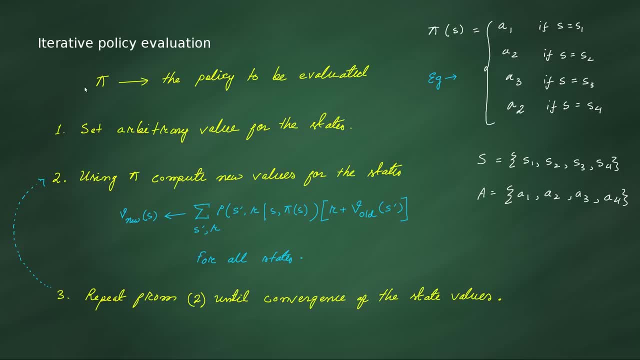 policy. so when I say it's a policy, it's just a table, like for a particular state. if your state is s1, then you apply action a1. if your state is a2, s2, then you apply a2. so it's like a table. so 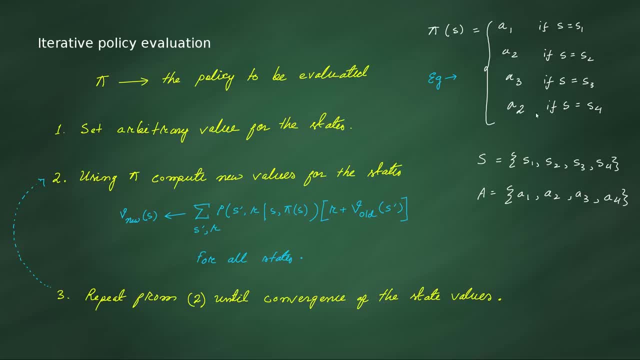 you randomly initialize this table. you can set like 0, 0, 0, 0, 0 action, or just left, left, left, left, and then this policy evaluation part, evaluate the values for all the states. so it evaluates the values for all the states. you remember? this is the equation for value function computation, the 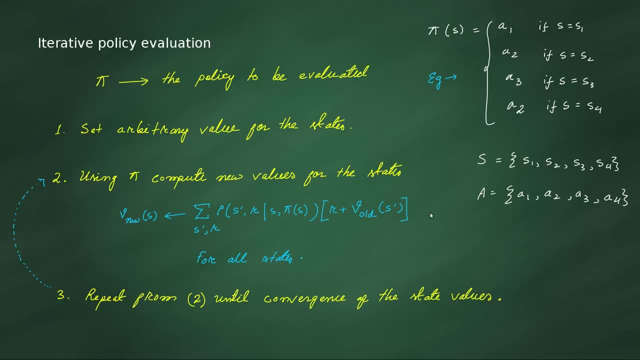 value, value computation. so this is the equation you remember. so it takes the old value of the states. all values are also like randomly initialized set, arbitrary, set arbitrary value for the states and you, using pi, compute new values for the states. so first you have to set the arbitrary states also. 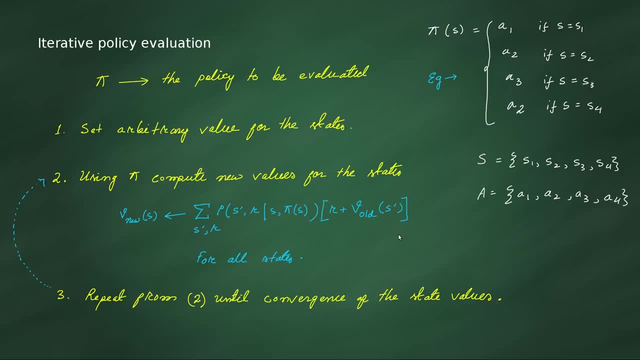 for the uh, for the environment. so we take, we can take 0, 0, 0 everywhere, or we can take one, one, one, one, one everywhere. whatever we want, we can take. so then what happens? using this equation, you update the values for the, for all the states, from the old values. from the old values, you update the values. 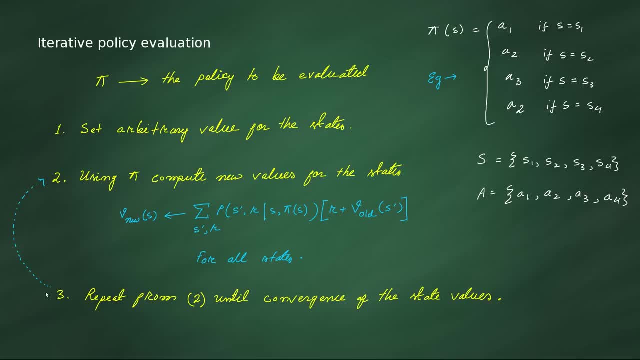 for all the states using the policy, and then you repeat the state. now, now you have updated, now it becomes the old value, and then you update the new value again using the currently updated values, so last updated values. so, uh, it's like this. it goes on a loop, again and again, and again, until you reach the convergence. the convergence is when 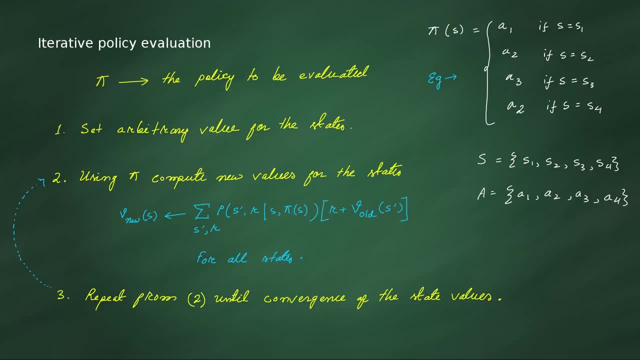 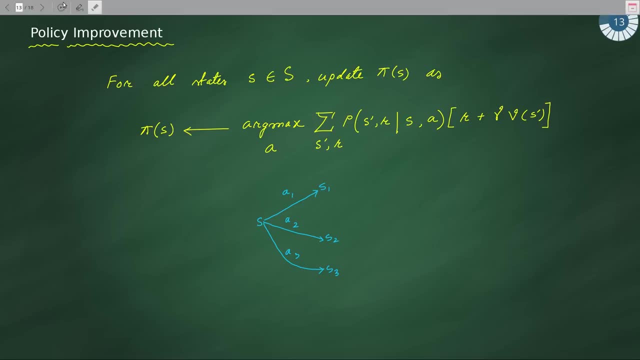 the values are not changing too much. so at that point you have to stop and you have to go to the policy improvement step. so what is policy improvement? so this is policy improvement in. policy improvement is not a loop, it's just one step. and policy improvement, what we do, we take the action. okay, we take the action that Maximizes. 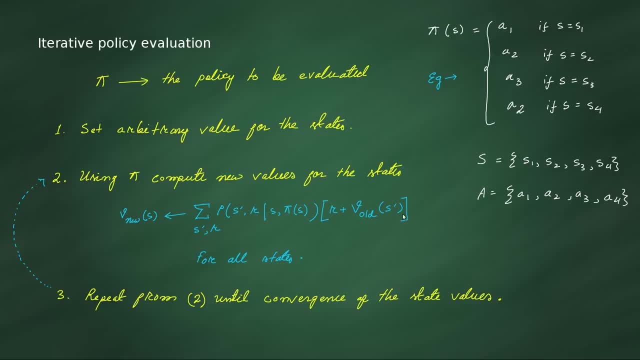 you update the values for the for all the states from the old values. from the old values you update the values for all the states using the policy and then you repeat the state now, now you have updated, now it becomes the old value, and then you update the new value again using the currently updated values, so last updated values. so it's like 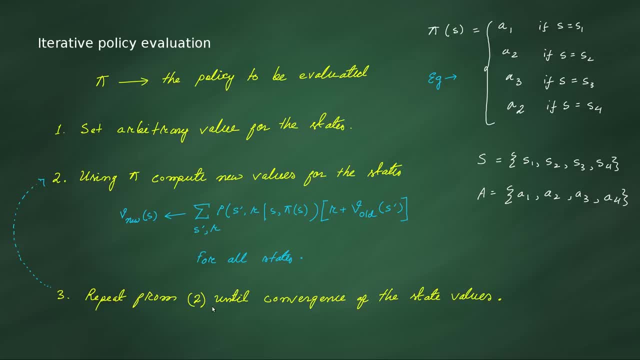 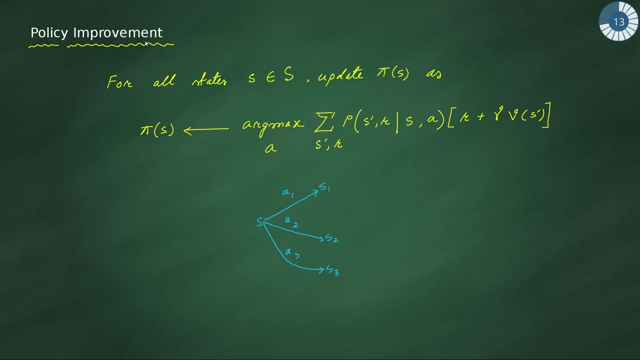 this. it goes on a loop, again and again, and again, until you reach the convergence. the convergence is when the values are not changing too much. so at that point you have to stop and you have to go to the policy improvement step. so what is policy improvement? so this is policy improvement in. policy improvement is not a loop. 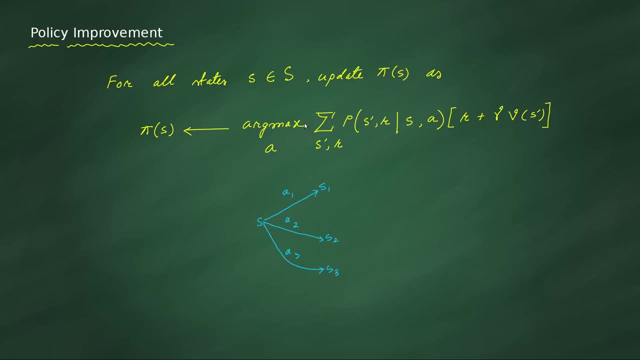 it's just one step in policy improvement. what we do, we take the action. okay, we take the action that maximizes this expression. and you remember what is this expression? it is the expectation of this term. the next reward plus discounted value of the next state. okay, this is the expectation of this term. we know the probability. that's why we're multiplying and 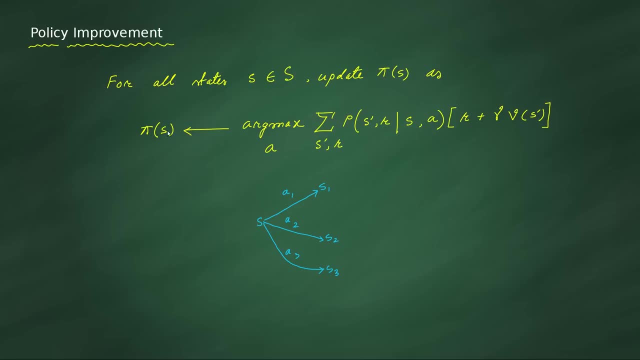 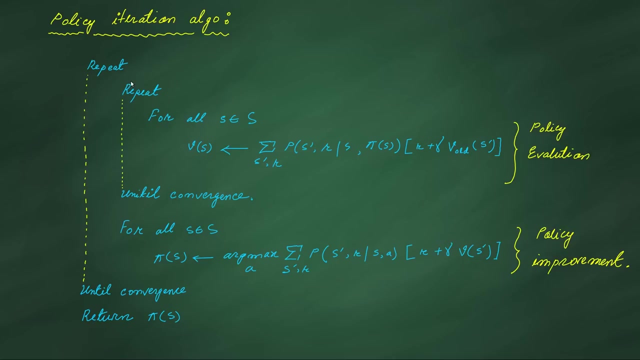 we are adding and we have to take the action, and this is the policy for this particular state. policy will give the action, and action is this one, this is the action and accordingly we update the table. let's see the complete algorithm in a proper way. so, policy iteration algorithm. so 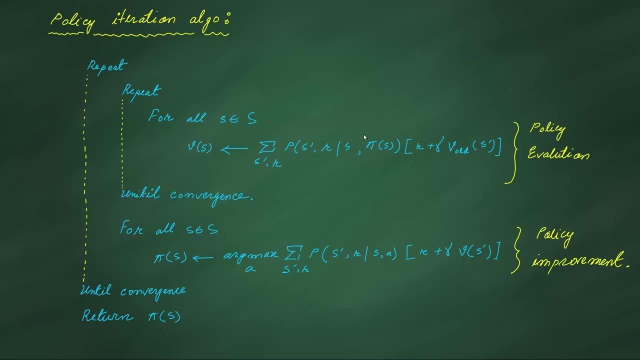 it has two loops. the first loop is the policy evaluation. we talked about it already. so it attributes the state values using the policy like this, and then, once it is converged, then this part, this policy improvement, takes the values of the states and update the policy and this outer loop. 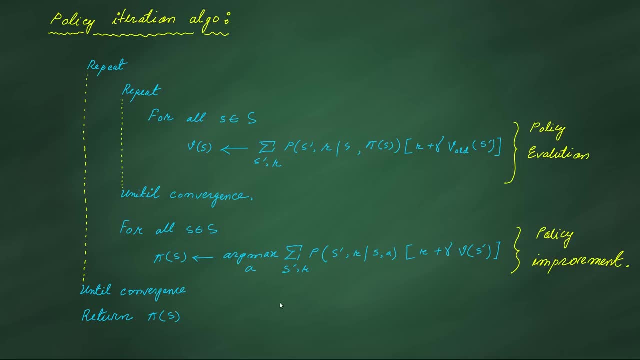 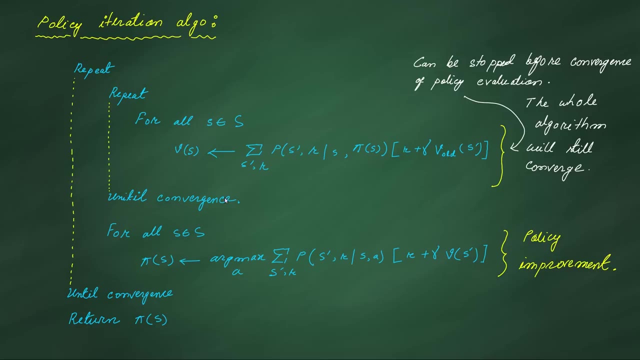 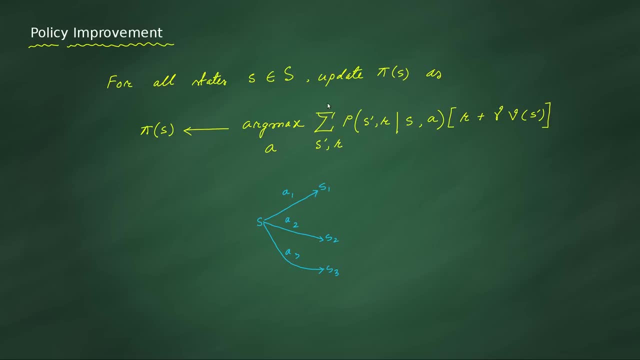 these expression and you remember what is this expression. it is the expectation of this term. the next reward plus discounted value of the next state. okay, this is the expectation of this term. we know the probability. that's why we're multiplying and we are adding and we have to take the action and this is the policy for this particular state policy. 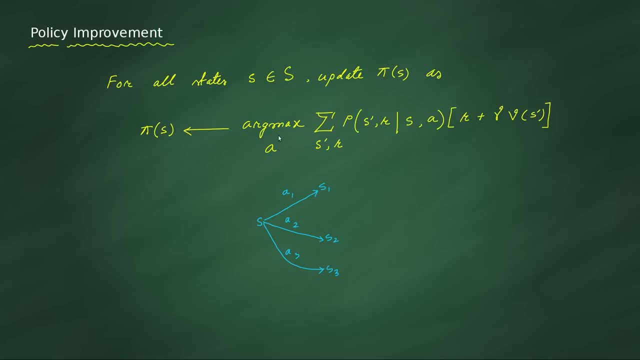 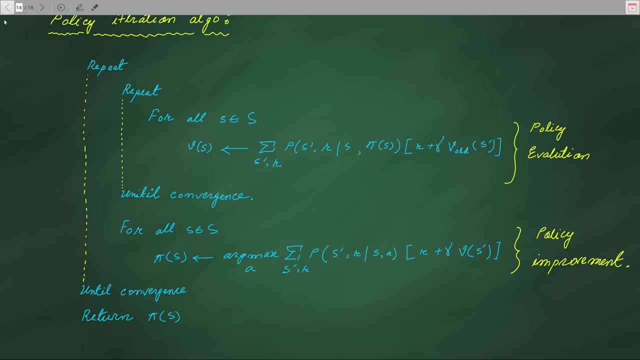 will give the action, and action is this one. this is the action and accordingly we update the table. let's see the complete algorithm in a proper way. so policy iteration algorithm. so it has two loops. the first loop is the policy evaluation, we talked about it already. so it computes the state values. 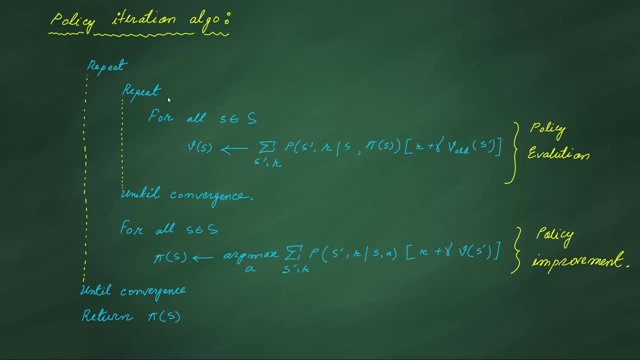 using the policy like this. and then, once it is converged, then this part, this policy improvement, takes the values of the states and update the policy, and this outer loop continues again and, again, and again until a stable value is reached. so now the question is here: you have to reach the 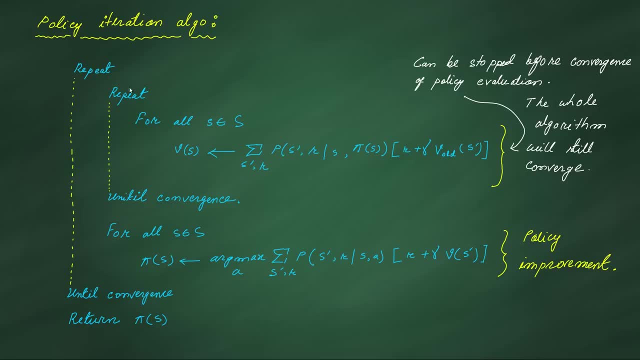 convergence. I told you like can we stop it before convergence, like can we do like two, three iteration of this and then go to this? and actually we can. we can stop this and this is called truncated policy evaluation. so we can truncate this like we can, like 10 iterations and we don't have to wait for. 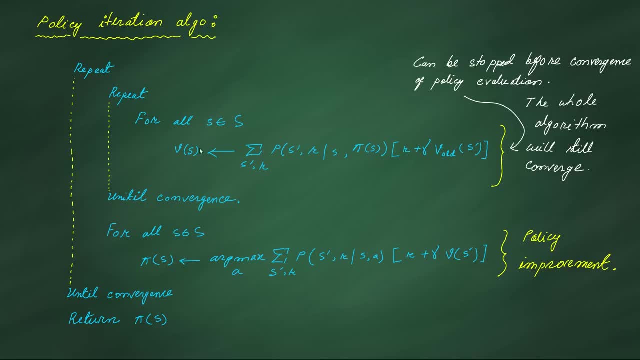 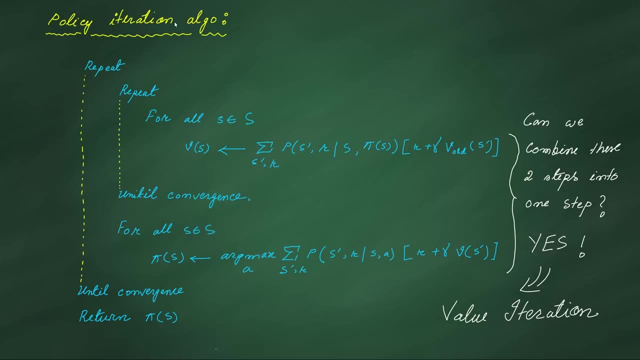 convergence till the. this algorithm will guarantee convergence to the optimal policy. so now can we close the conversion and then we can do like two, three iterations of this and then go to this and up this two parts of policy iteration into one. so we have two parts right. one is this loop and one 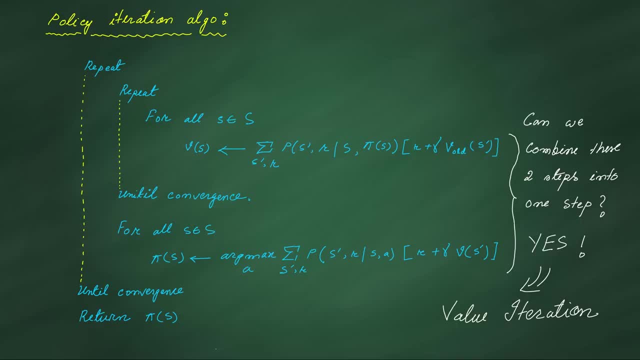 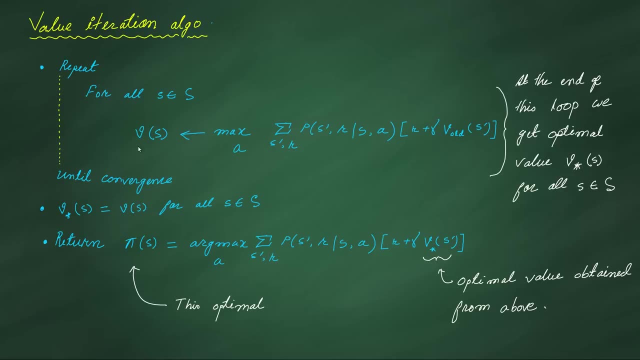 is this. so can we join them together? and we can actually, and this is called value iteration. so let's see what is value iteration? so this is value iteration. so we are not now evaluating the value with respect to a policy, like in policy iteration. we are computing the values. from the old values, but we are going to compare the entire new view and then we are taking the values which are going money value. so, other than the multiple, we apply, say transform, and we take the values as буду positive as possible. we are goal and cooked experiments. we are executing the values which year these things sixteen days for six weeks. man does so. this is how we 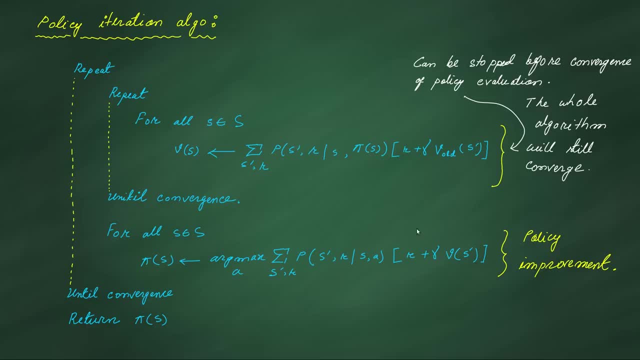 like two, three iteration of this and then go to this and actually we can. we can stop this and this is called truncated policy evaluation. so we can truncate this like we can, like ten iterations, and we don't have to wait for convergence till the. this algorithm will guarantee convergence to the optimal. 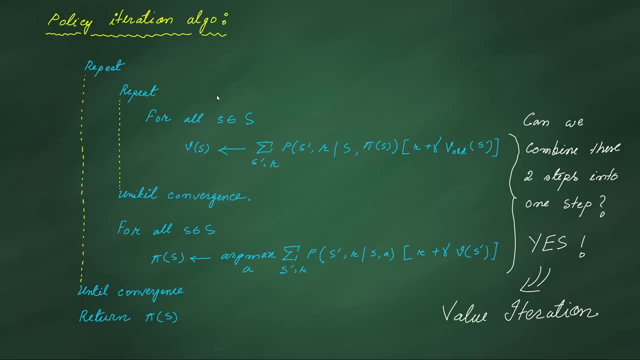 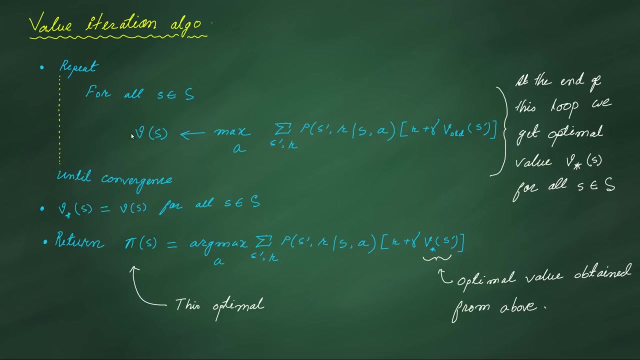 policy. so now can we club these two parts of policy iteration into one, so we have two parts right. one is this loop and one is this. so can we join them together? and we can actually, and this is called value iteration. so let's see what is value iteration. so this is value iteration, so we are not now evaluating. 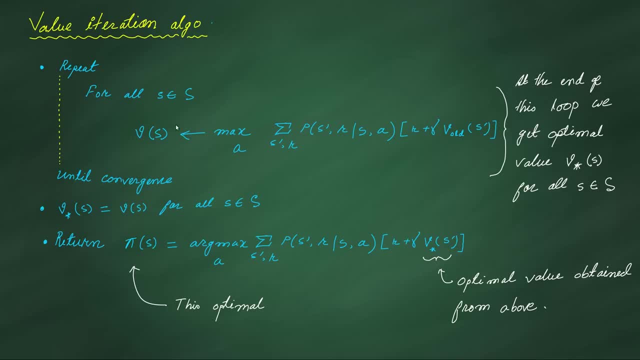 the value with respect to a policy. like in policy iteration, we are computing the values from the old values with respect to a policy. now we are not computing it with respect to a policy, but how we are computing it. we are computing the next value, the new values of a new value of a state, using the action that maximizes. 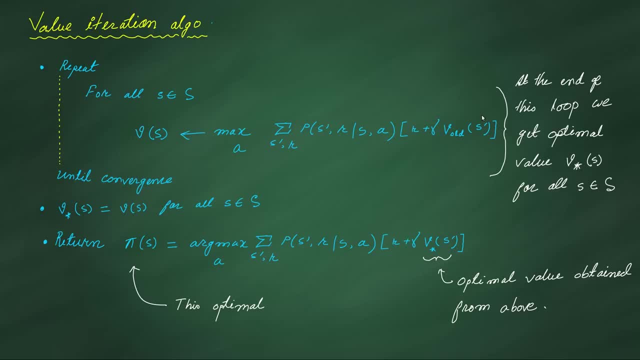 this term and this whole term is the expected total discounted reward. yeah, so once this loop is converged- that means the value of the states are not changing too much- then we can say that we reach the optimal value of the states, or very close to the optimal values for the states. and then, once we reach this value, 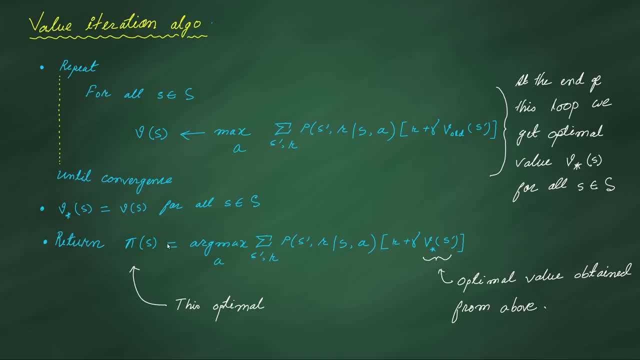 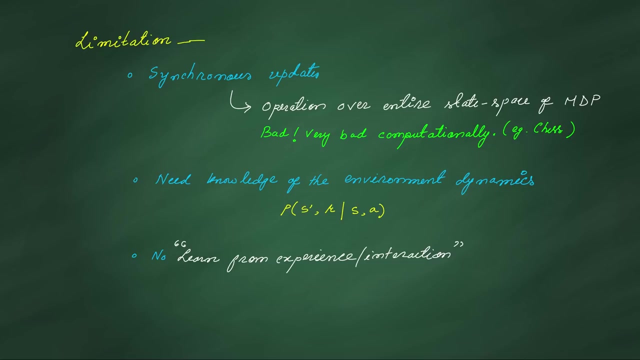 we can simply compute the policy in one step. this is the action that maximizes this term. it's the expectation of total discounted reward. so this is the value. iteration algorithm is very simple. so what is the problem with these two algorithms actually, if you think that we are actually doing it synchronously? if we have very huge state space in the 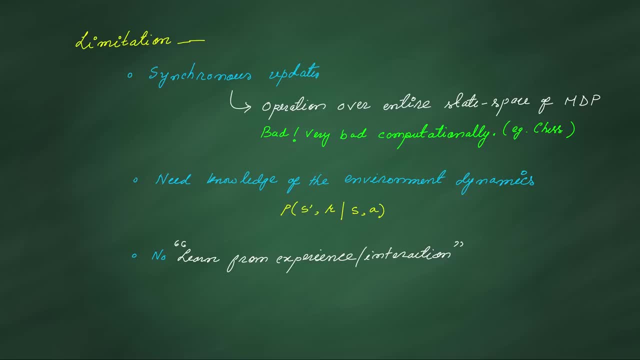 environment. then we have to update all the values together, like in one loop of the algorithm, like policy evaluation. then we are actually updating, or even value iteration, we are updating all the values of the states in every loop, right? so this is very computationally expensive and we cannot actually focus. 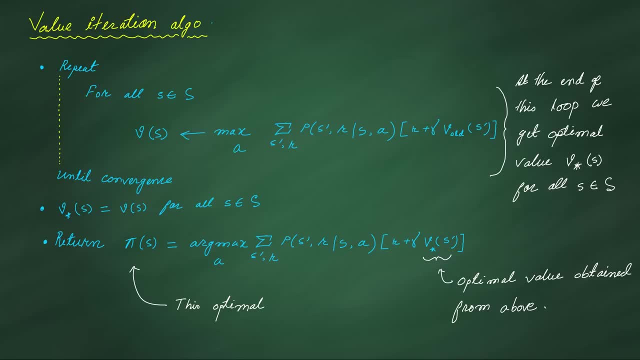 with respect to a policy. now we are not computing it with respect to a policy, but how we are computing it. we are computing the next value, the new values of a new value of a state, using the action that maximizes this term, and this whole term is the expected total discounted reward. 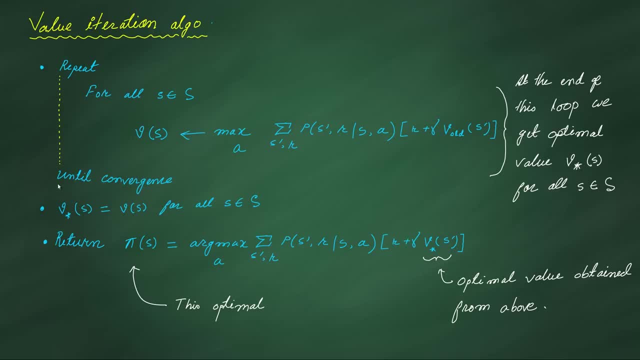 yeah, so once this loop is converged- that means the value of the states are not changing too much- then we can say that we reach the optimal value of the states, or very close to the optimal values for the states, and then, once we reach this value, we can simply compute the policy in one step. this: 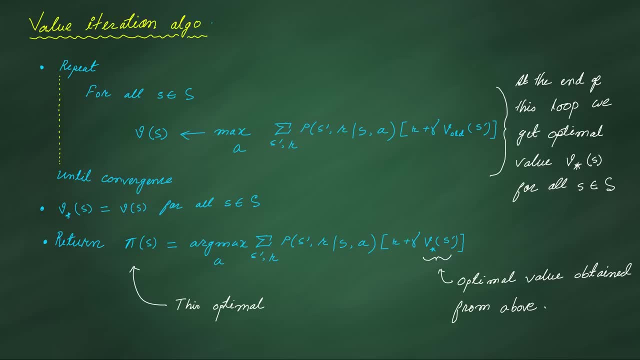 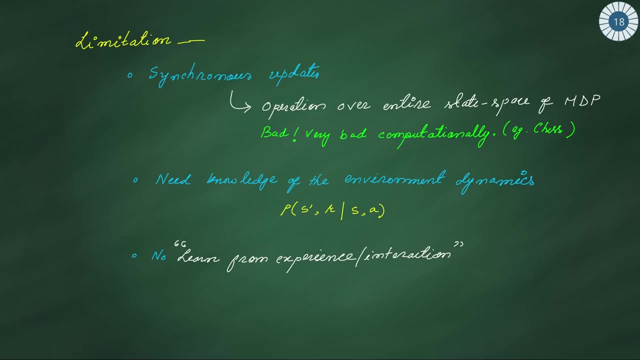 is the action that maximizes this term. it's the expectation of total discounted reward. so, again, we are not computing it with respect to a policy, but how we are computing it with respect to this is the value iteration algorithm. it's very simple. so what is the problem with these two? 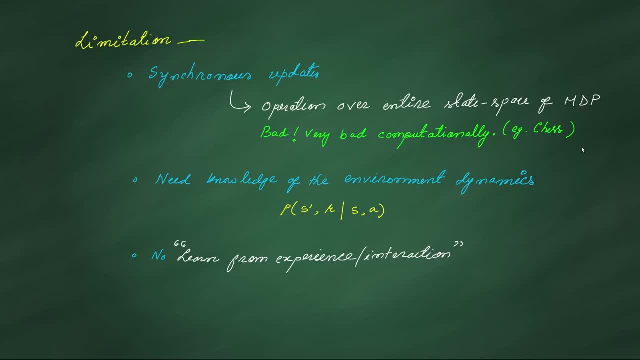 algorithms. actually, if you think, then we are actually doing it synchronously. if we have very huge state space in the environment, then we have to update all the values together, like in one loop of the algorithm, like policy evaluation. then we are actually updating, or even value iteration. we 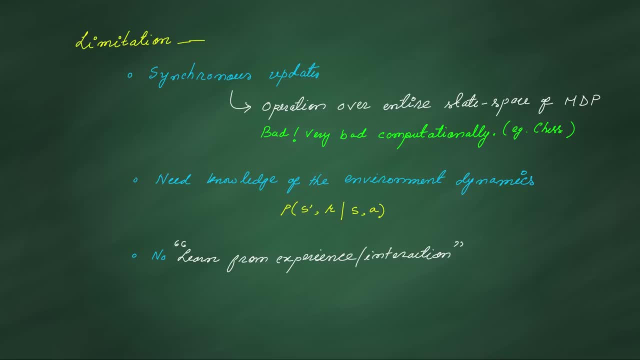 are updating all the values of the states in every loop right, so this is very computationally expensive and we cannot actually focus in way in the relevant region of the state space. if we know this is the relevant region of the state space, maybe goal is there, maybe. 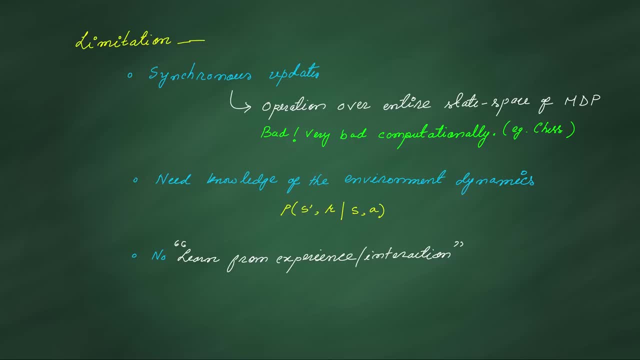 we know a bit about the environment, then we cannot focus this algorithm towards those regions. we have to do updates for all the states, right? so this is not efficient, so need then second the problem. the second problem is we need the knowledge of the environment dynamic, okay, so we need this probability distribution, okay. so since we need this, we cannot use it like 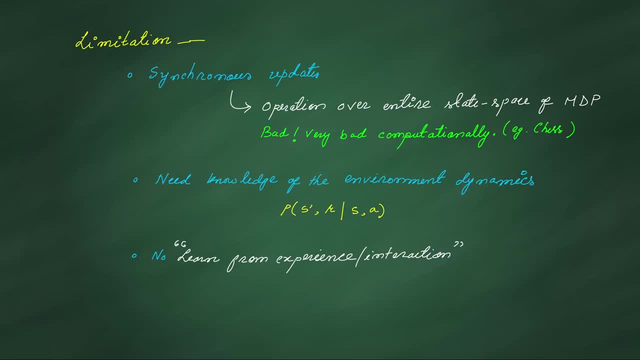 a learn from experience or learn from interaction way. we cannot let the agent do something in the environment and from that we learn something and accordingly we update the policy. we cannot do it with this algorithm, so in upcoming videos we will study about something called Monte Carlo approach.